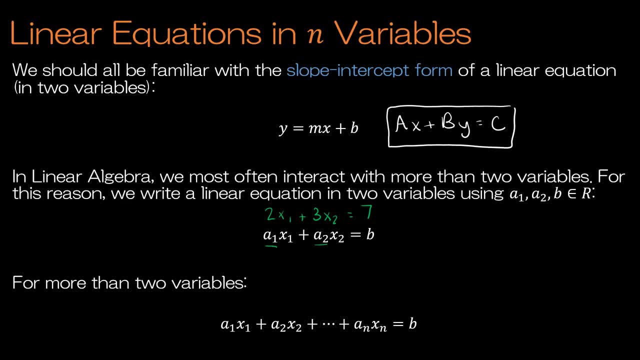 Again, for more than two variables, we would just continue that pattern- a1x1,, a2x2, an xn and so forth- and we would not be able to solve a linear equation. So again, just remember that we're going to be focusing on two variables. 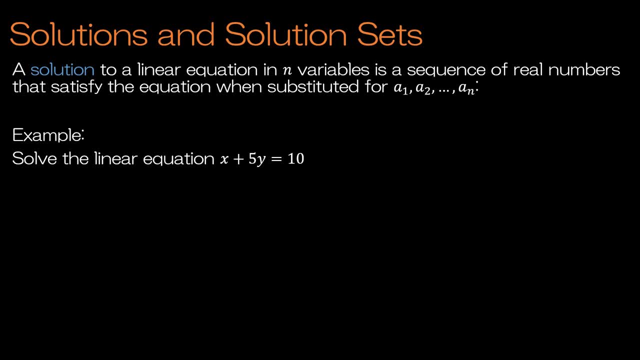 and a1 equals some real number, b. Now we want to take a look at how to find a solution to a linear equation in n variables. And what's one thing new that we're going to look at- and possibly you've studied this before in calculus 2 or 3,. 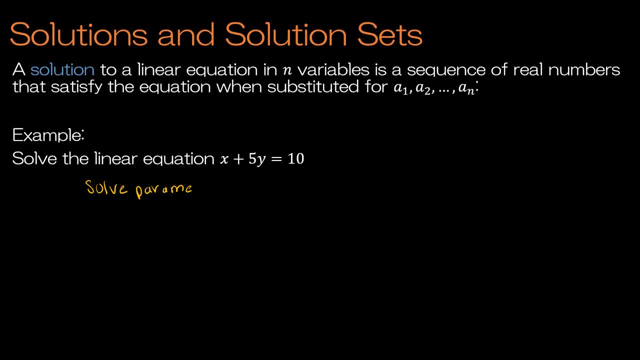 but if you haven't, don't worry, we're actually going to solve this parametrically, which means we're going to solve. Before we do parametrically, let's just look at how we might solve this normally. So normally, we would just say: oh, let's make an X- Y table. 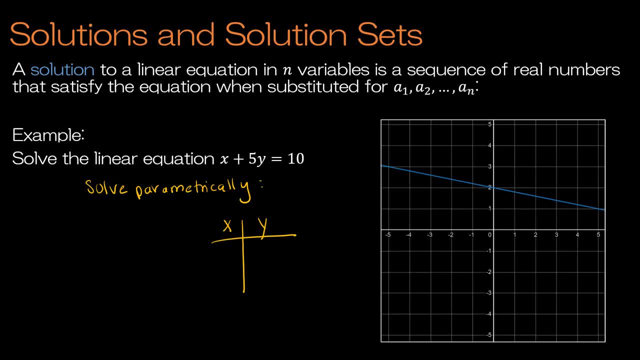 and then we can plot a graph that has all of the points on it, And that's okay, and that's kind of what we're going to do now. But what we're going to do is we're actually going to set X equal to some expression. 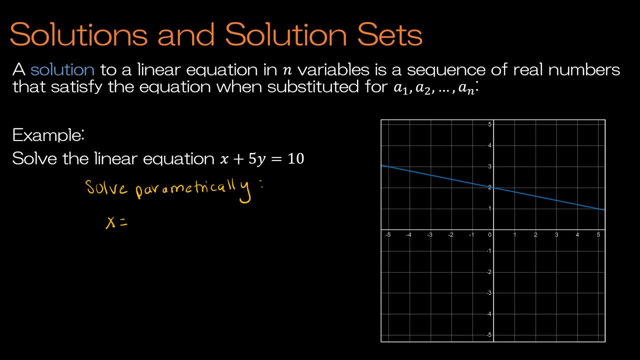 based on the parameter of T. So we're going to make T our parameter And that just is going to be the. it's just basically another variable that changes. So we can set some limits to our parameter: an upper bound, a lower bound, and so forth. 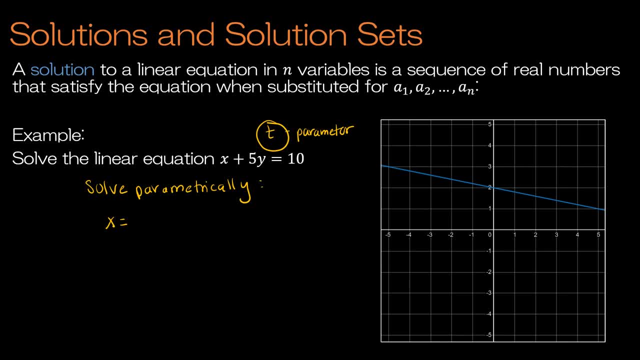 But everything is now going to be based on T. So to get X by itself, I'm just going to do some normal algebraic manipulation. I get X is equal to 10 minus 5Y, And Y is then going to be: 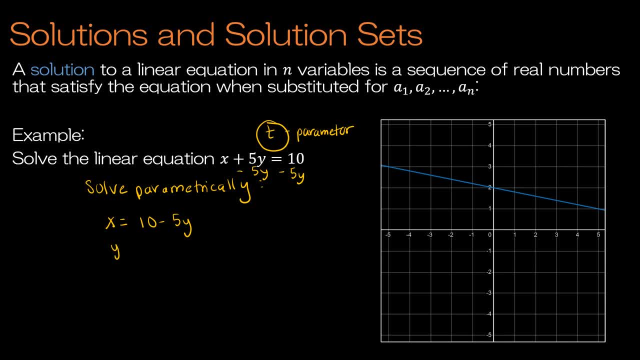 my free variable. So think about the independent, dependent variables. We're saying Y is independent and X is dependent on Y, But now we're going to write this parametrically. So we're going to say: let Y equals T, T is the parameter. 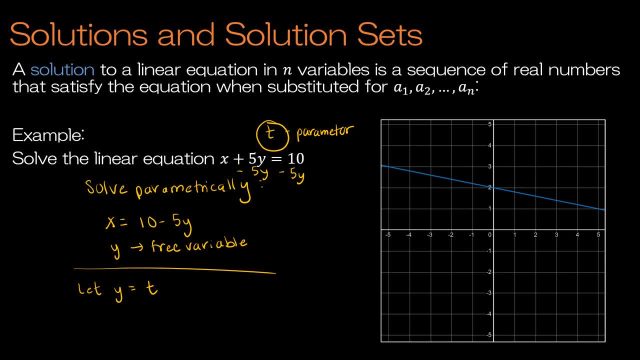 And so T is going to be whatever, sorry, Y is going to be whatever We set for, T, And X is going to be 10 minus 5T. So, again, this is the correct solution. The graph doesn't change, but it would be based on the value of T. 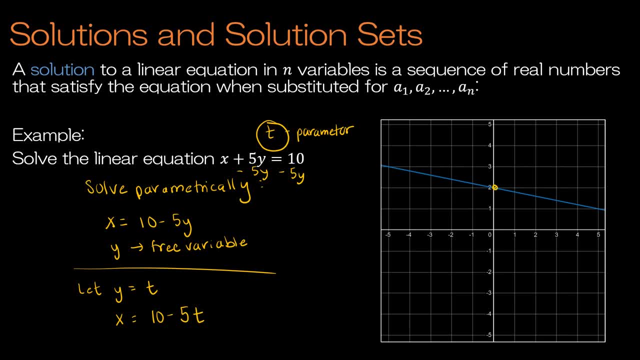 So here this ordered pair is still the point 0 on the X, 2 on the Y, But that means it's also where T is equal to 2.. So that's how we would find that. So that is using the parameter of T. 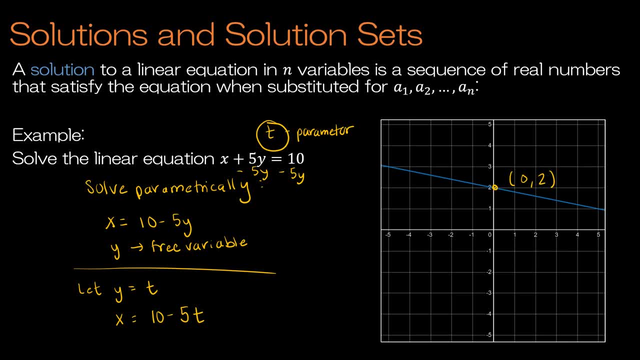 It's still going to give us the same graph, but solving parametrically is going to be something that we do quite often. Let's go back to the topic of free variable, So keep in mind that it would be possible in this case. 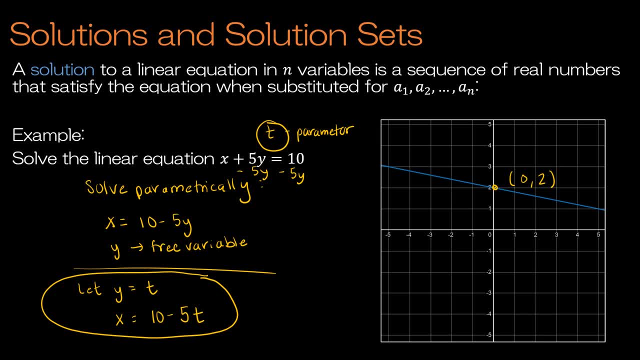 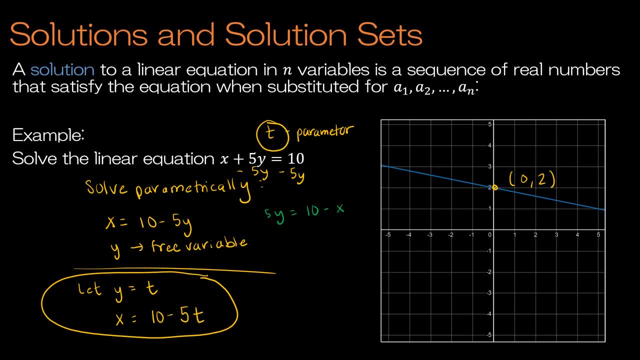 Well, I could have said: let 5Y equal 10.. So you have 10 minus X. Therefore Y by division by 5 would be 2 minus X over 5, or 1 fifth X. Therefore Y by division by 5 would be 2 minus X over 5, or 1 fifth X. 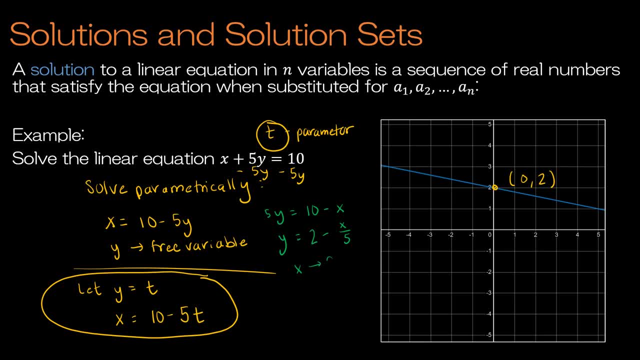 And then X would be a free variable. Would that be the exact same thing? And the answer is yes. Typically we're going to use whatever free variable is easiest to find And typically it's going to be a variable that's shorter than a variable. 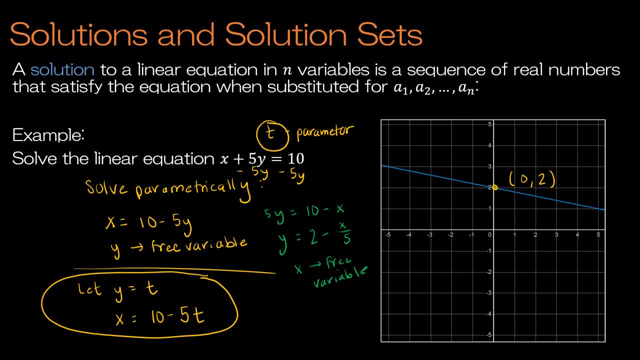 going to not be the x variable. that is free. but you'll see, as we work more and more with parametric equations and with linear systems, exactly what a free variable can do for us. Now that we understand how to find a parametric representation, let's do so for an equation. 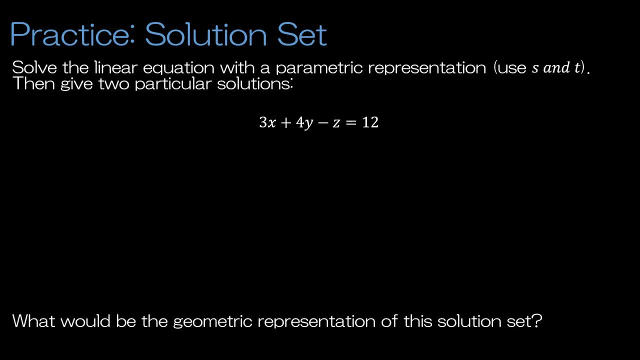 involving three variables. Now, keep in mind I could have just as easily written this as 3x1, 4x2 minus 1x3 equals 12, and we would be doing this exactly the same way. So how am I going to solve this? Well, I'm going to start by getting a variable by itself. So let's. 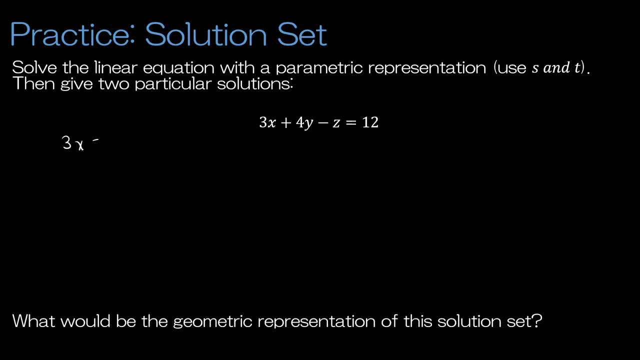 isolate 3x. 3x is equal to 12 minus 4y plus z. So I've just shifted the 4y and the z to the opposite direction. So I've just shifted the 4y and the z to the opposite direction. 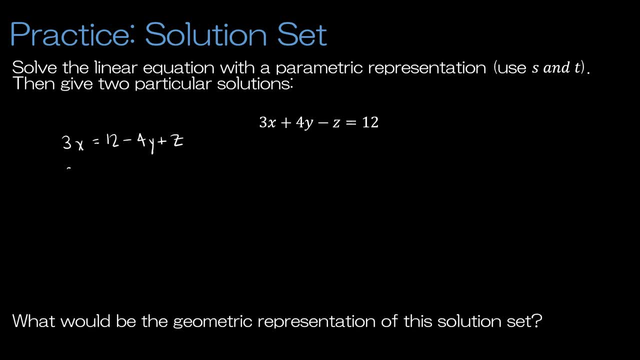 Of course changing the signs. Then I'm going to divide everything by 3.. So 12 divided by 3 is 4.. Then I get 4 thirds y and I get 1 third z. So what's my parametric solution? 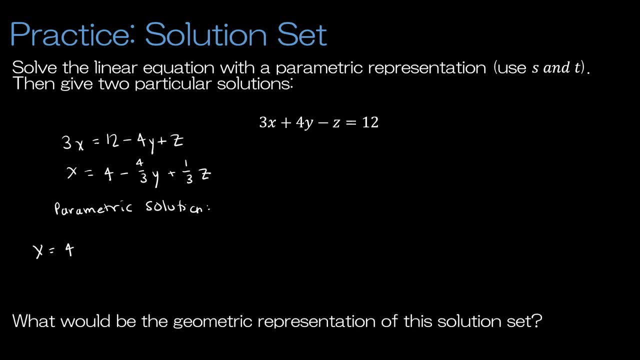 That x is equal to 4 minus 4 thirds x. So we're now going to use s and t because y and z are both going to be our free variables. So 4 thirds s, 1 third t, where y is equal to s and z is equal to t. 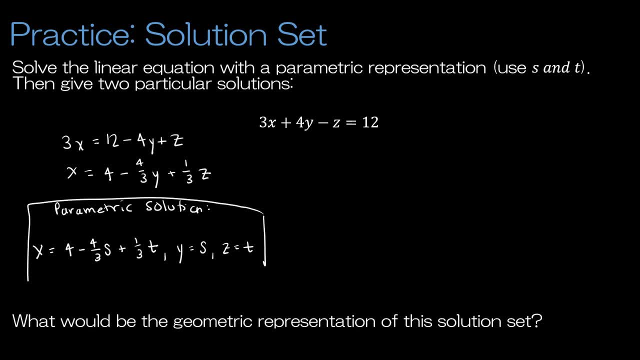 This is my parametric solution: Two free variables. x is reliant upon the value of those free variables. It also asks us to then give 2x2.. 2 particular solutions. So that's the very easy part If we need a particular solution. 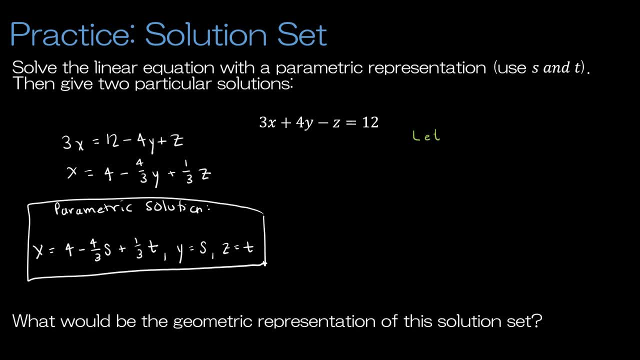 essentially, I'm just going to assign a value for s and assign a value for t, which is our two free variables, s and t, And then I'm going to find x based on that. So I'm going to say x is equal to 4 minus 4 thirds times 0 plus 1 third times 0,. 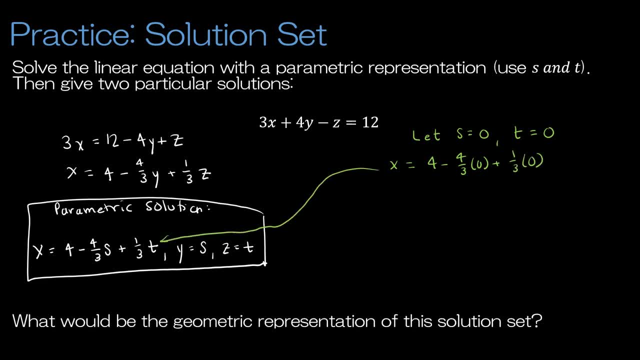 so I'm just using this equation and replacing with 0, s and t, And that would just give me 4.. So one solution would be: x is 4, y is 0, z is 0. And another solution I can find the same way. 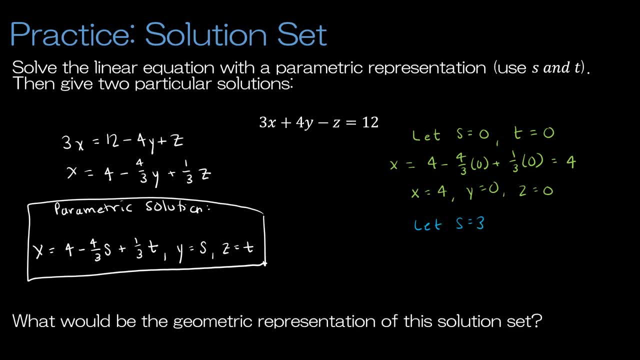 So I'm going to let s equals 3 and t equals 0.. So x is equal to 4.. So I'm going to let s equal to 4 minus 4 thirds times 3, plus 1 third times 0, which gives me 4 minus 4 thirds times 3 is 4, which is, and then minus 0, which is 0. 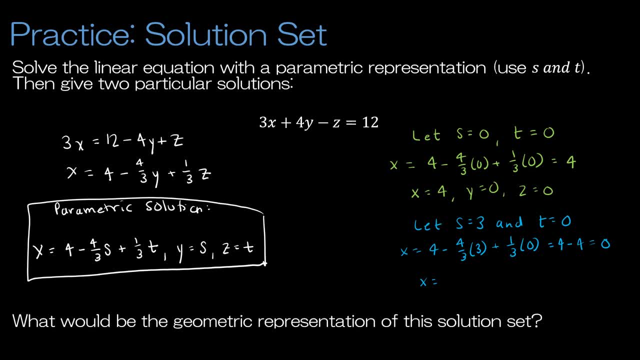 So another solution would be 0 for x, 3 for y and 0 for t for z. Now the last question says: what's the geometric representation of this solution set? Hopefully we know, because we have 1,, 2,, 3 variables. 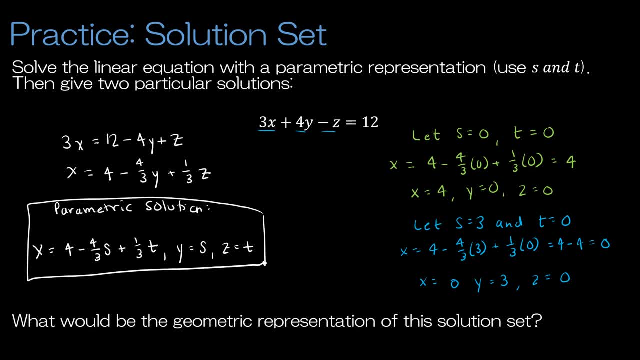 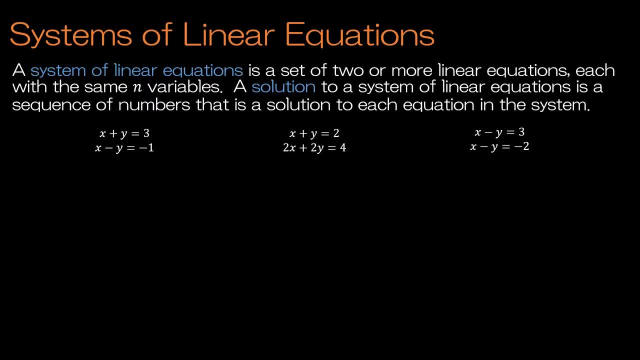 Our geometric representation would be a plane in three dimensions using the x, y and z axes. Now it's no fun just to talk about one linear equation. So let's talk about a system of linear equations, because that's where all the fun happens. 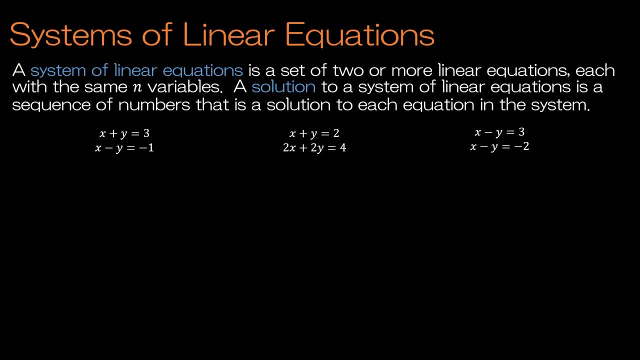 Now I'm going to be using just a set of two linear equations and two variables to demonstrate what our possibilities are. Obviously, as we study more into linear algebra, you will be having more variables, more equations and so forth, But for now it's important to understand the basics. 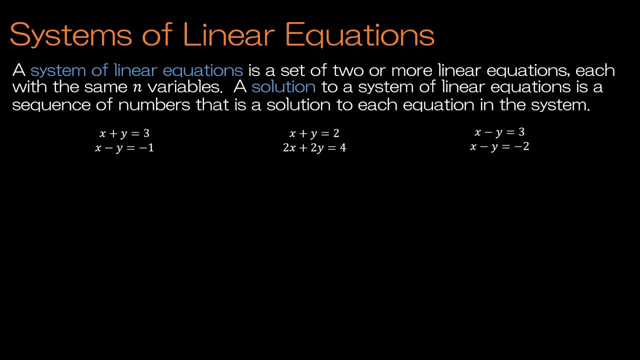 What are the possibilities when you have a linear, a system of linear equations, You can either have one solution. So here let's say I was solving this by adding together 2x plus plus y. minus y gives me 0,, 3 plus negative 1 gives me 2, so I get x equals 1.. 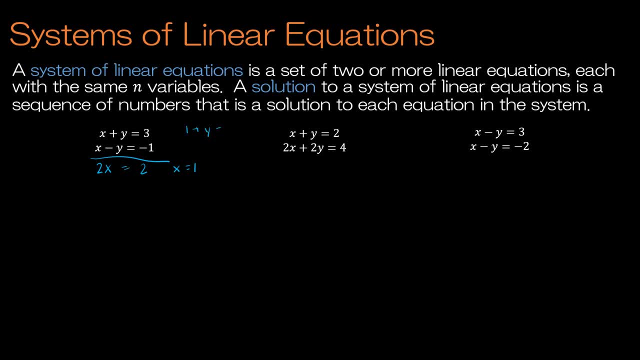 And then I would plug 1 back in to say: 1 plus y equals 3, so y must be 2, so my solution is 1 comma 2.. That's what happens when I get one solution: They can cross at exactly one point. 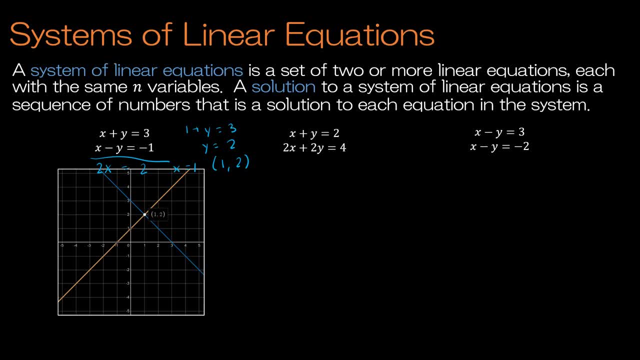 Now I could do the same thing with the next equation, but hopefully I can see that if I took the first equation by 2, I would actually have the exact same thing as the second equation. So my second possibility, my first possibility, is that I have just one solution. 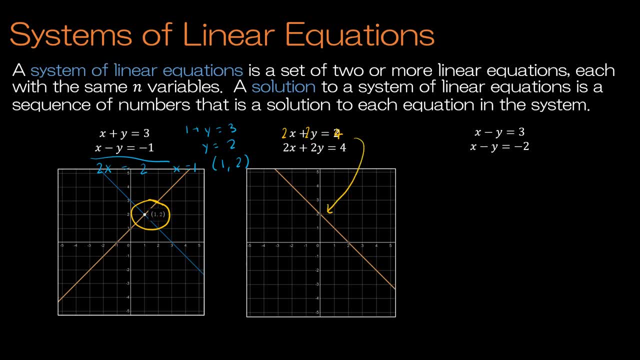 My second possibility is that I have the same exact equation two times, which means everywhere the first equation happens, the second equation also happens, so it's really two lines on top of one another. So I'm going to have as many solutions as there are points on the line, which is an infinite number. 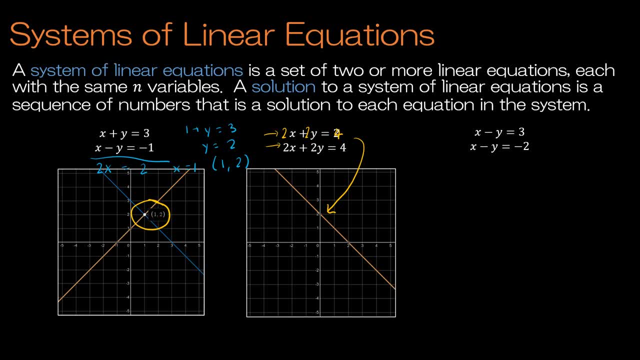 And for my last one, let's say I subtract these equations: x minus x gives me 0,. negative y plus negative y- I'm sorry- minus negative y gives me 0, and 3 minus negative 2 gives me 5.. 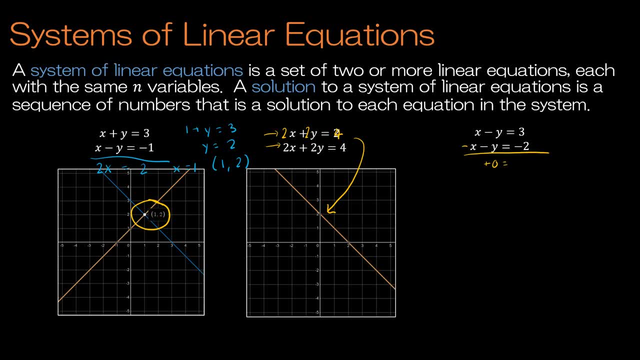 Well, that doesn't work right. 0 can never equal 5.. So if I get an equation like that, I can see that these two are parallel. Are these ever going to touch each other? No, Because they're parallel and will be until eternity. 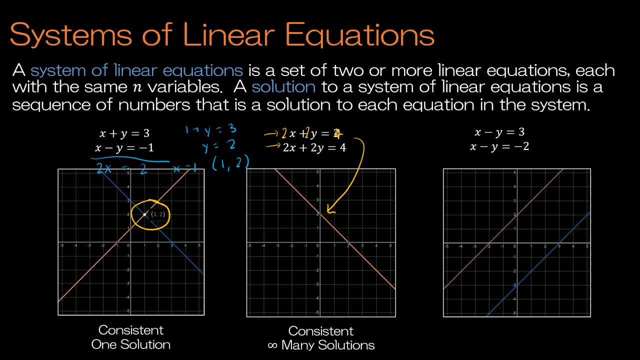 So we can either have a consistent one-solution equation, consistent infinitely many-solutions system, or an inconsistent no-solution system. So notice: if we do have a solution, it's considered consistent and if you don't have a solution, it's considered inconsistent. 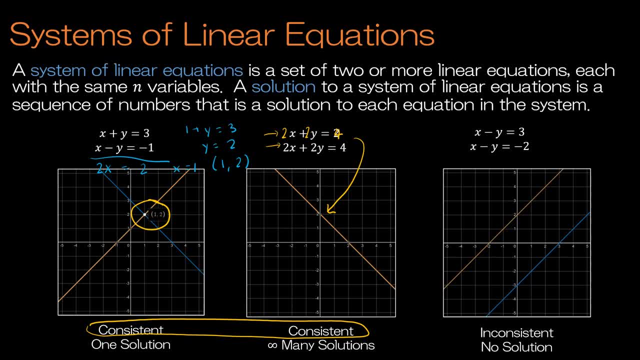 There are two ways to have a consistent system. You can have just one solution, where that one point where two lines, or three lines, or four lines or so on meet, or two planes and three planes, and so on. Or you can have infinitely many solutions if all of the lines or planes are exactly the same. 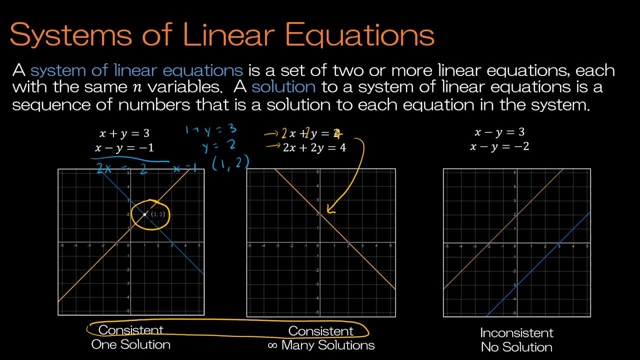 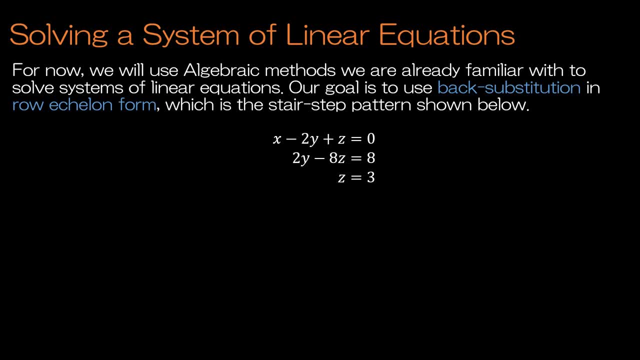 Or you can have an inconsistent system with no solution. I'm certain that we've all studied before how to solve a system of linear equations by substitution, elimination or graphing. That should have been a prerequisite that you studied in Algebra 1, Algebra 2.. 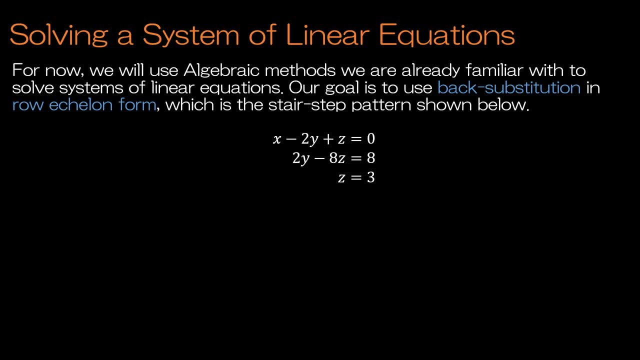 So for now we're going to fall back on those methods for solving this system of linear equations. Now, this one happens to have three variables and we're just going to use something called back substitution And a new term to throw in. there is row echelon form. 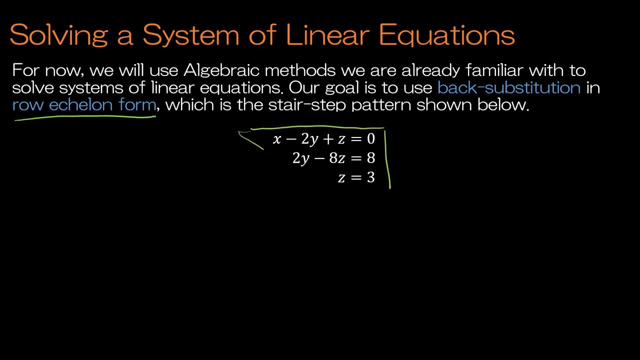 This system is in row echelon form because, as you can see, it's sort of a stair-step pattern. One of them has three variables, The next has two, The next has one and so forth, So I'm doing this with just three equations. 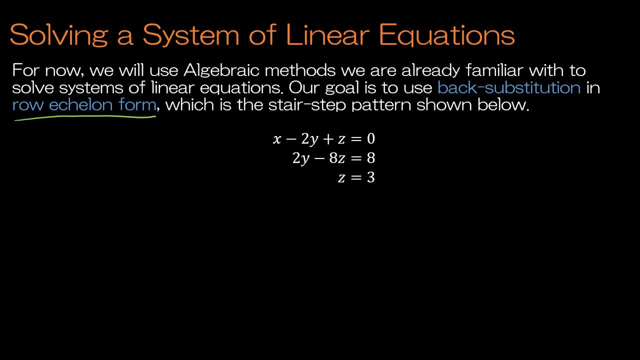 You could do it with more, But solving a system in row echelon form is actually pretty straightforward, because I already have z And in order to solve for the other variables, I'm just going to start at the next stair up. So I know that z is 3.. 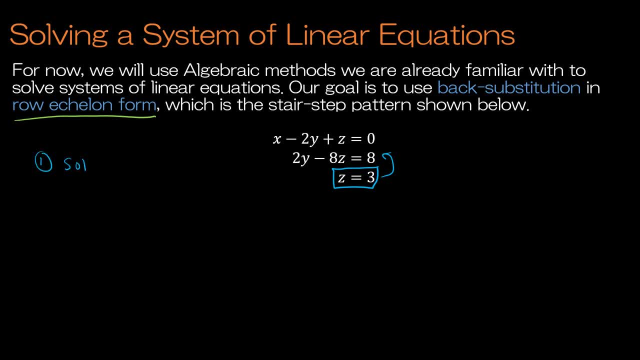 And then my first step, then, is to solve for y, Which means I'm going to take that second equation. So 2y minus 8z- but instead of z I'm plugging in 3, is equal to 8.. 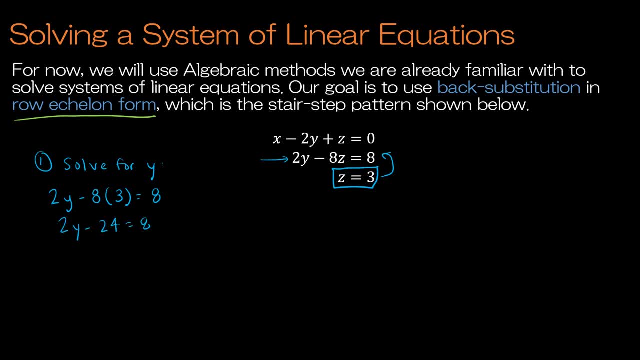 So 2y minus 24 is 8.. Add 24 to each side. I find that y is 16.. Next step, step two, solve for z. So I already. I'm sorry for x, I already know y. 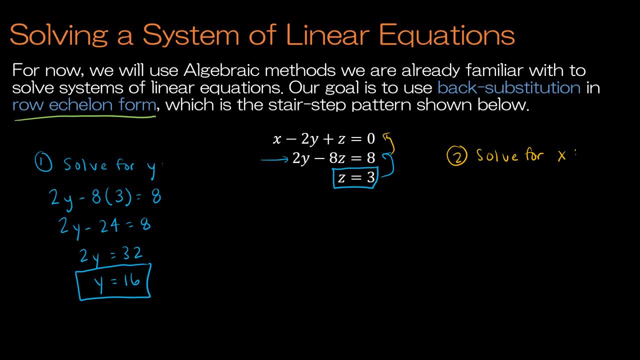 I know z, So I'm going to now move to the next stair-step up. I'm going to say x minus 2y Instead of y, I'm replacing 16.. Plus z, which is 3, must equal 0.. 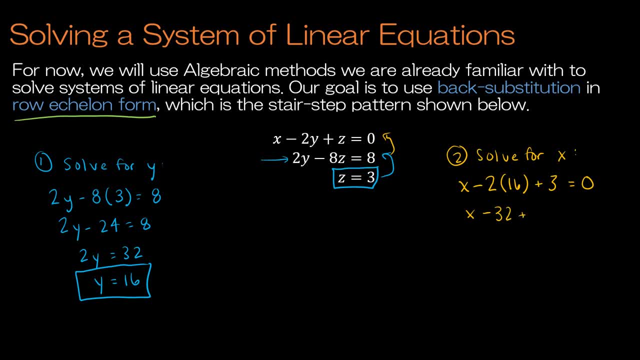 So x minus 32 plus 3 is equal to 0.. I end up with: x minus 29 is equal to 0. Add 29 to each side, x is 29.. And then, of course, the final step is just to. 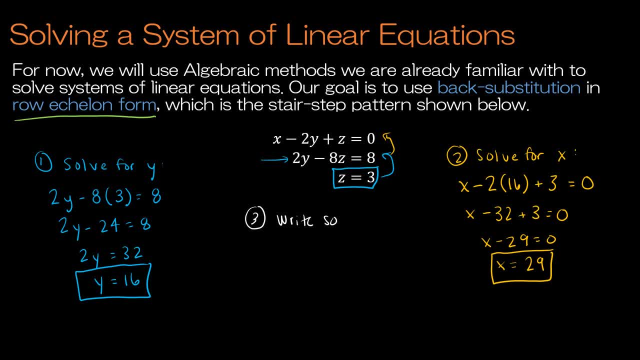 write your solution. So my solution is x is 29.. y is 16.. z is 3.. So you might be asking: can I just write that as 29,, 16,, 3?? Yes, you can. I'm just going to be very clear that x is 29,, y is 16,, z is 3.. 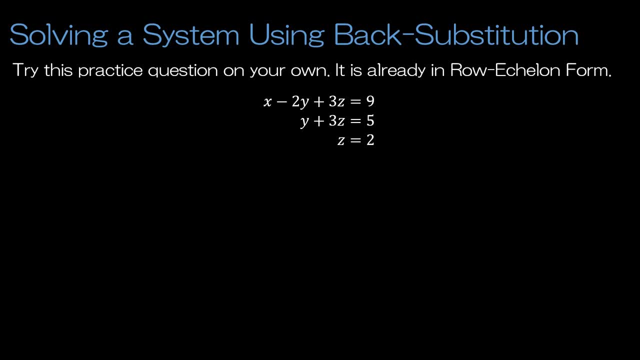 Here's another question. This one is- it's already in row- echelon form, So I would like you, if you could pause this question and try it on your own first, before I go through the solution with you And when you're ready. 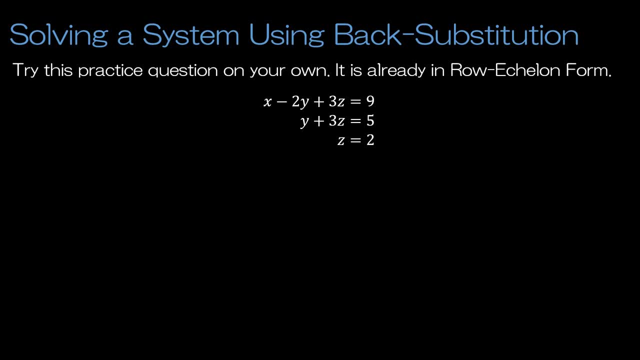 just go ahead and press play to see how you did Again. I already know that the solution for z is 2.. So I'm going to start by taking y. So this is step 1, find y. y plus 3 times 2 is equal to 5.. 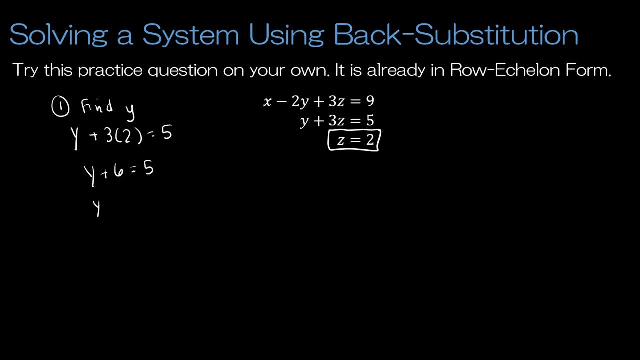 y plus 6 is 5.. y is equal to negative 1.. And then step 2, I'm going to find x. So I know that x minus 2 times y plus 3 times z is equal to 9.. So x negative 2 times negative 1 gives me plus 2.. 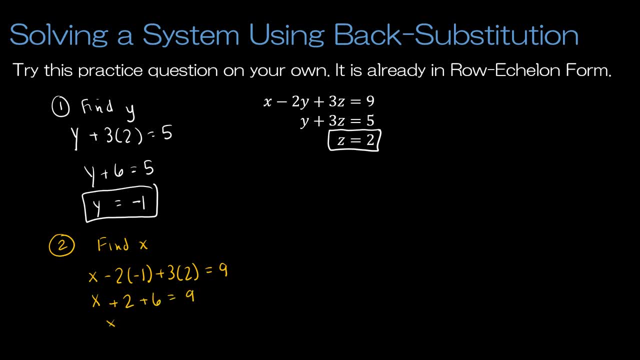 Plus 6 is equal to 9.. x plus 8 equals 9.. And then x must be 1.. So my solution- oops, I meant to change color there. My solution: x is 1,. y is negative 1,. 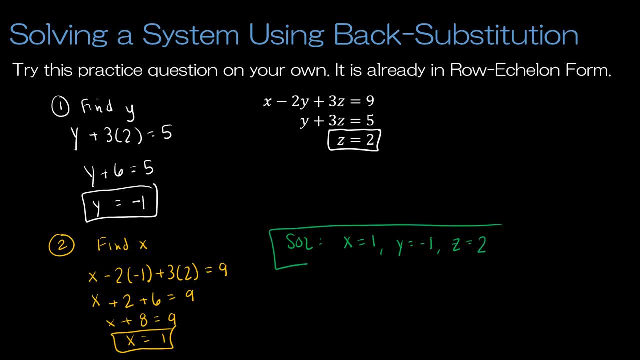 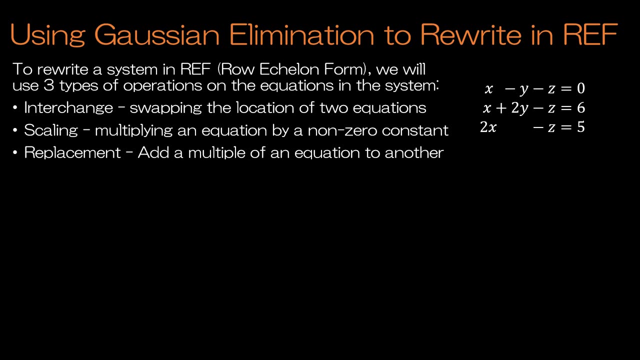 z is 2.. And again, this is a system that has just one solution. What we want to do now is take a look at a system of linear equations that is not already in row echelon form. So let's take a look at a system of linear equations that is not already in row echelon form. 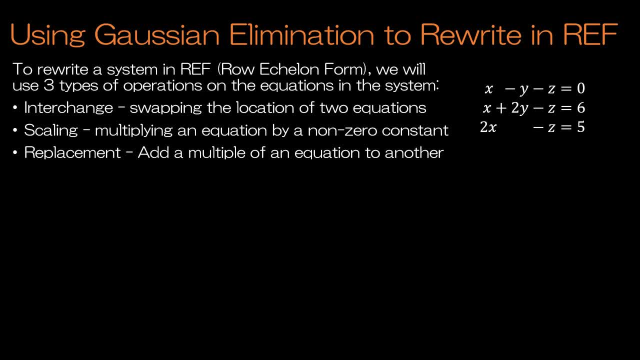 It's going to be very important that we know how to take a system of equations and turn it into row echelon form. You might be tempted to skip over this, but this is really the solid foundation that you're going to need, because we're going to continue with these, what are called row operations. 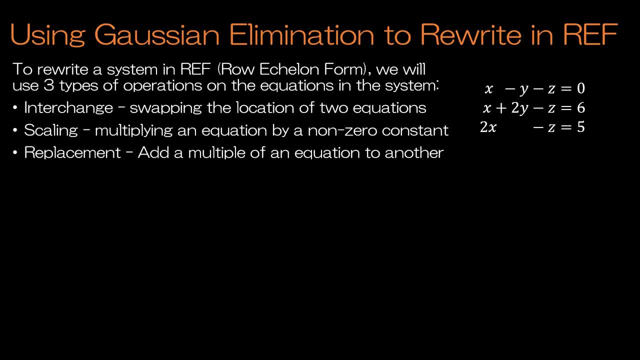 even when we're working with matrices. So this is obviously not dealing yet with matrices, but we're going to be using the same system. So when we are writing, when we are writing an equation in row echelon form, we only have three operations that are able or available for us to use. 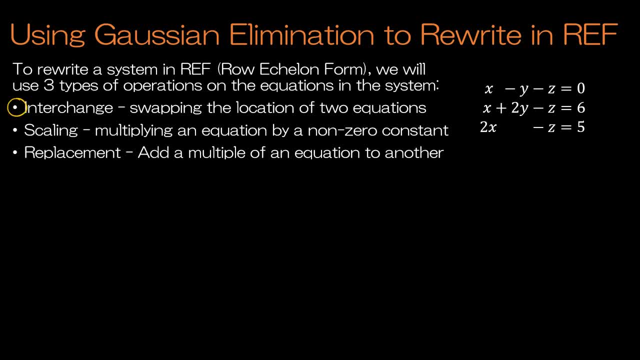 The first is an interchange, And in an interchange we're essentially just going to switch the location of two equations. So, for instance, we know that we want the first equation and I'm going to call this row 1, row 2,. 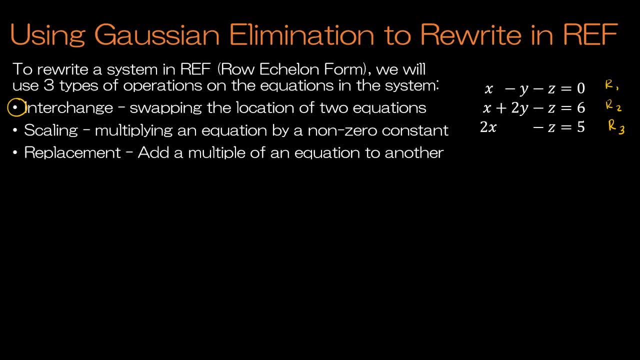 row 3.. In the first equation I have x, y, z. But what if it was just: z equals 0?? Well, I know, in row echelon form I need that to be the last equation, So I would just use an exchange or an interchange. excuse me, 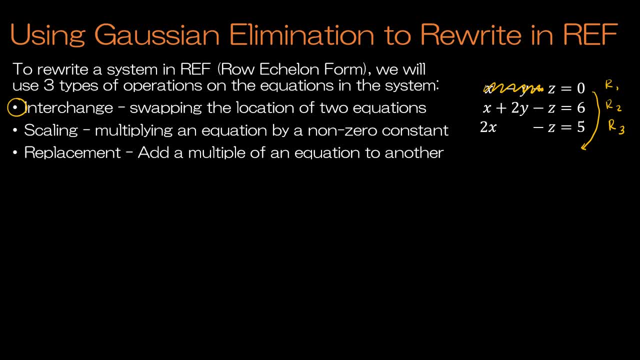 to swap the location of 1 and 3.. So I would move the location of those two. Now, if you're going to use an interchange, which doesn't happen super often, it's one of the probably the least common of the three. 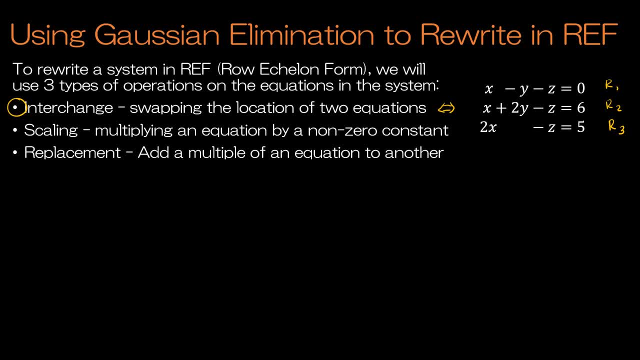 you're going to use basically an equal sign with an arrow on each side to show that you're interchanging two rows. The next row operation is scaling. Scaling is, let's say, I had 2x minus 2y minus 2z. 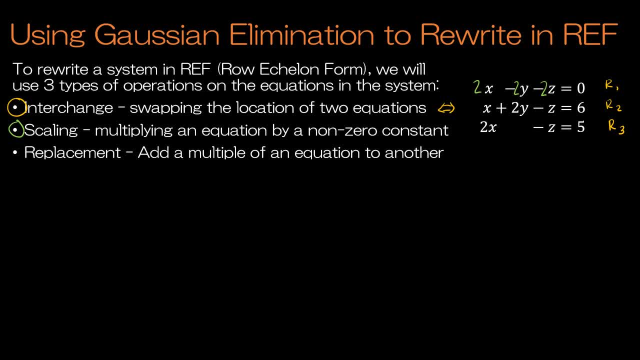 Well, it would be very easy for me to get x by itself by just dividing by 2.. But now I can't divide, I can only multiply. So instead I would simply multiply by 1 half. So if you're going to use scaling, 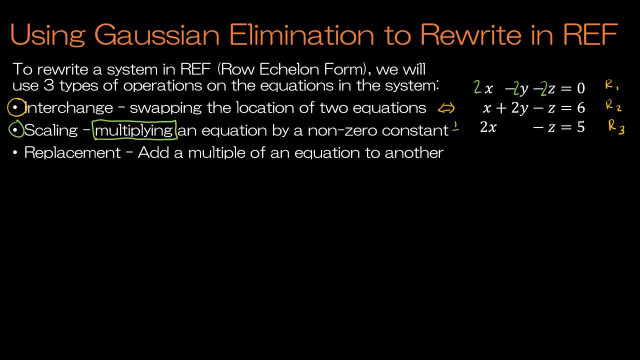 we would just show whatever that scalar is and then times the row that you're going to be using. So I would take 1 half row 1 to be my new row 1.. And then the last one is replacement. Now, this one is the most common. 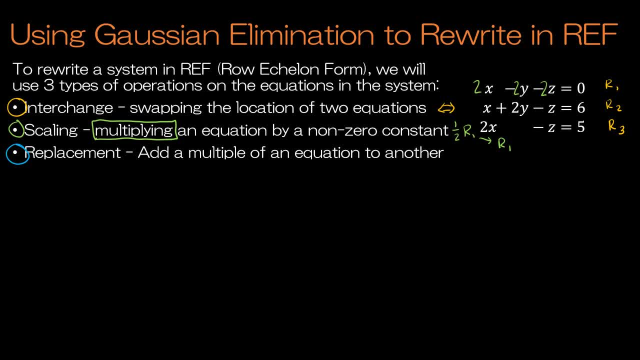 And when we replace, we're taking a multiple of an equation and adding it to another equation. So, for instance, if I were taking row 2 times negative, 2 times row 1 plus row 3. To be my new row 3.. 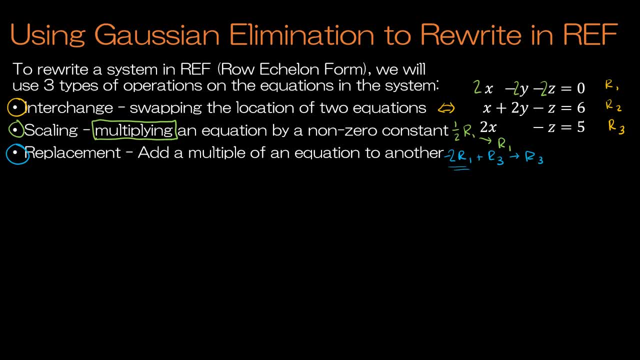 So notice, I'm taking a multiple of row 1. Which would give me negative 2, positive 2, positive 2.. And then, if I was adding it to row 3, that's going to get rid of that x. So those are my three options. 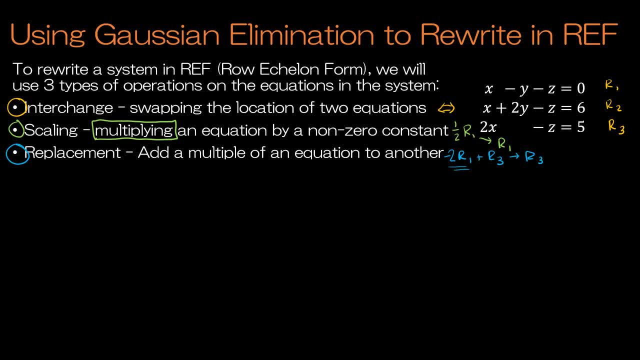 Now we're going to work through this one together fairly slowly, So if you're already familiar with all of this, feel free to skip forward, But I want to make sure that everyone has a solid foundation, because this is going to help you to be successful. 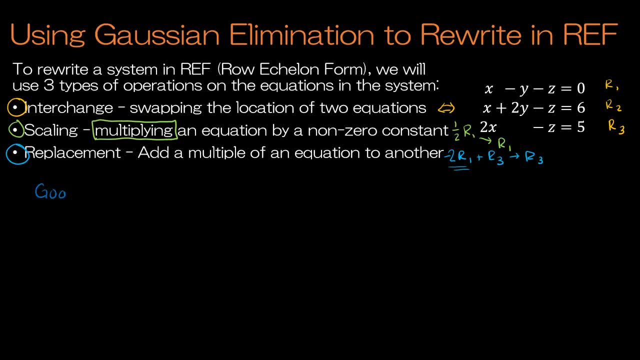 in this course. So here's my goal. My first goal is to eliminate the x's in row 1,, I'm sorry, in row 2 and row 3.. Because I have x, y and z already in row 1.. 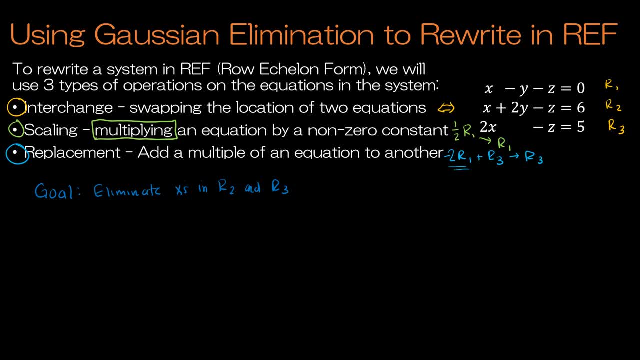 And now I want only row 1 to have the x. So the first thing I'm going to do- and I'm going to get rid of all of this other stuff that I've drawn just to make sure that everything's clear- What I want to do is: I want to be able to 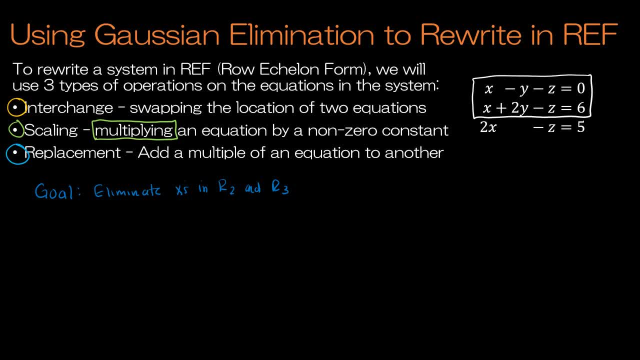 somehow combine these two to eliminate the x in row 2.. So it makes sense to me. And just a disclaimer here: you're going to do a lot of mental math. So if you're not so good at the mental math, get yourself a piece of scratch paper, because I'm not going to. 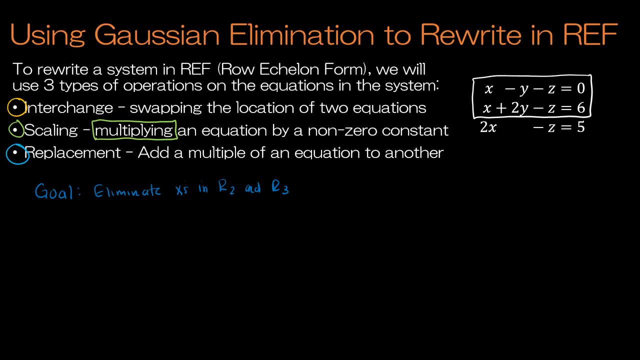 write out all of the things that we're going to do. So if I want to get rid of the x here, I would take that first row times negative 1.. And then, by adding them together, I would end up with negative x plus x, which is 0.. 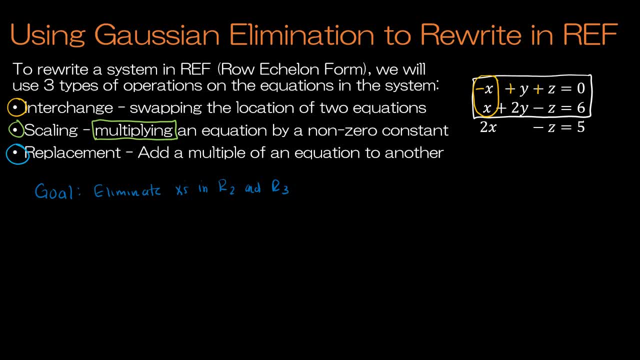 So I would end up with basically y plus 2y, which is 3y. So here let me just show you exactly what we're doing: I'm taking negative row 1,, I'm adding it to row 2, and I'm going to put that in the place of row 2.. 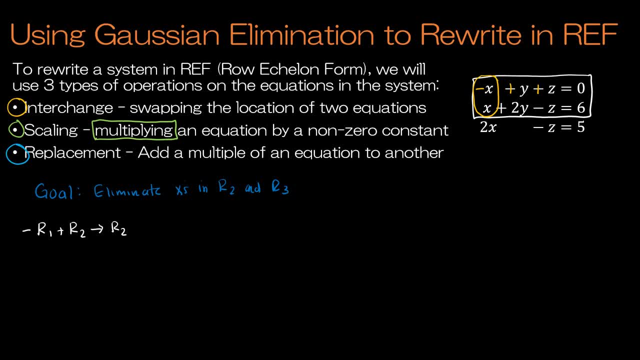 So I'm replacing row 2 with negative 1, row 1 plus row 2.. Now what's left after I do that? Well, I didn't do anything to the first row. Now you might be saying: well, yes, you did. 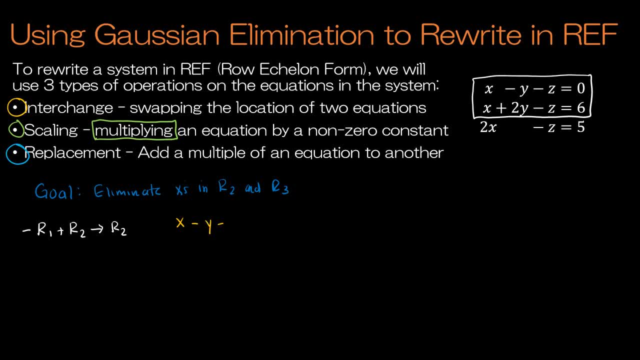 You took it times negative 1.. I did, but only the only reason I did that was to get rid of the x in row 2.. So I'm not actually changing row 1. Row 1's remaining the same. Then I'm going to do something to it to help me get rid of row 2,. 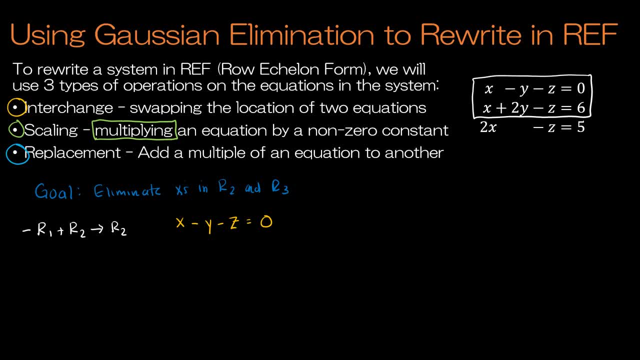 but I'm actually. that's not going to be a permanent change, It's just a temporary thing. So now, what happens with row 2?? Well, I took row 1 times negative 1.. I'm adding them together, I get 0.. 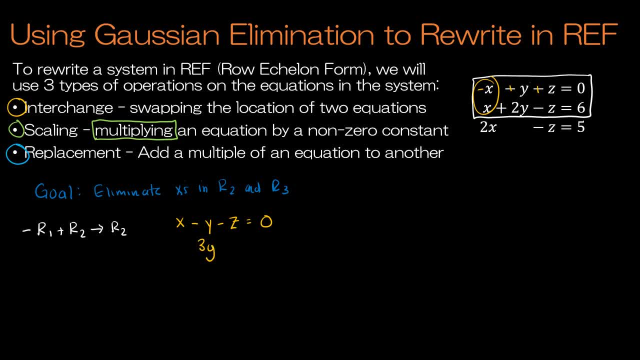 I get y plus 2y, which is 3y, And I get z minus z, which is 0,. right, So I have plus 0. And then equals 6, because 0 plus 6 is 6.. 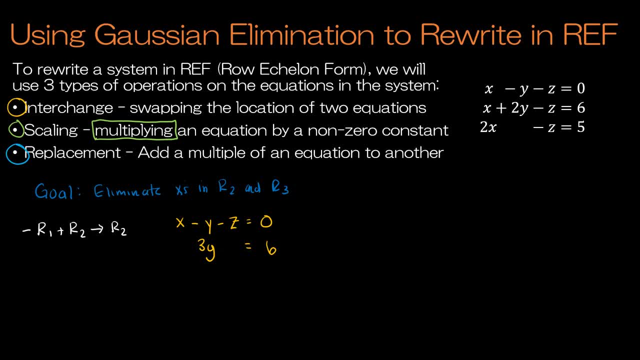 Okay, Now what's with the third row? Well, I haven't done anything to that yet, So this is still: 2x minus z equals 5.. Now I want to get rid of x in row 3.. How do I do that? 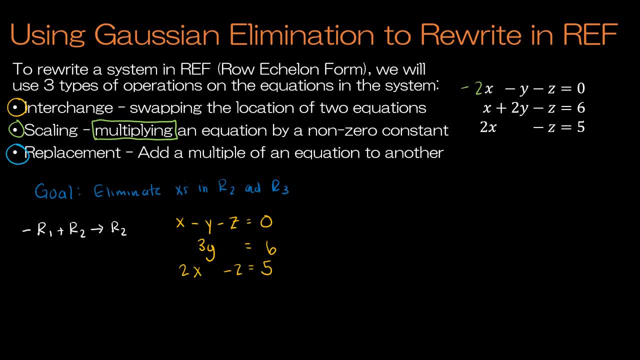 Well, if I took negative 2 times that first row- so again negative 2 times that first row- and added it to the third row, I could get a third row, a new third row that doesn't have an x in it. 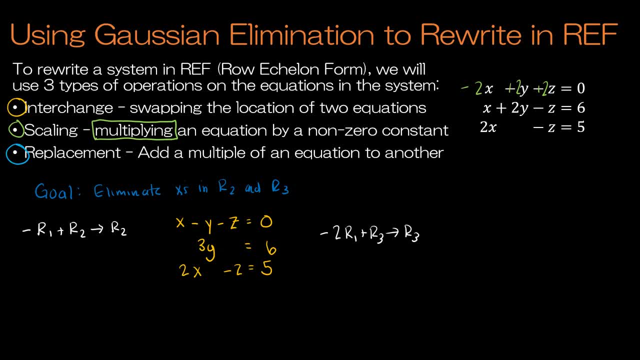 So what is my remaining system of equations? Well, I still have x minus y minus z equals 0, because, remember, this is just a temporary change, It doesn't change it permanently. I have 3y equals 6,, so I haven't done anything to the second row in this step. 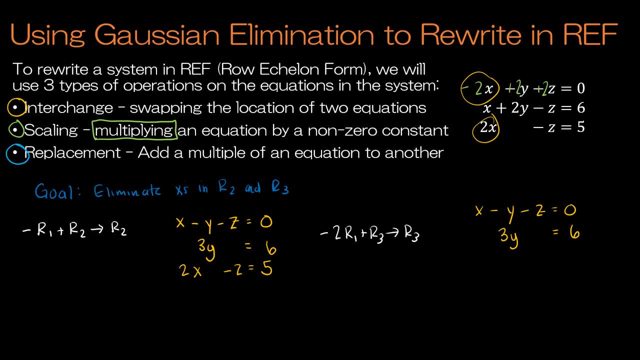 And then I'm going to have negative 2x plus 2x, which is 0.. I have negative 2y plus 0,, which is 2y, And then I have 2z and negative z, which gives me z. 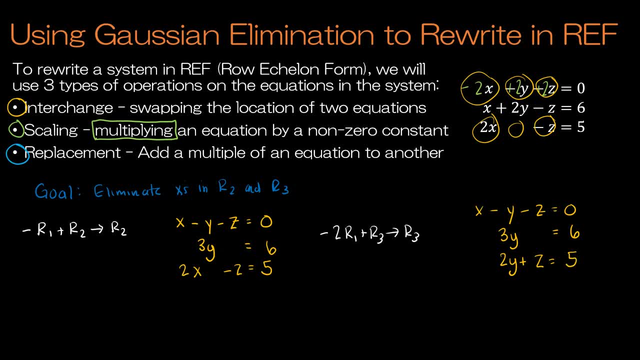 and 0 plus 5, which is 5.. So this is where I am so far. Now, what do I want to do next? I want to eliminate the y in the third row because the first row, remember. I want all of the values. 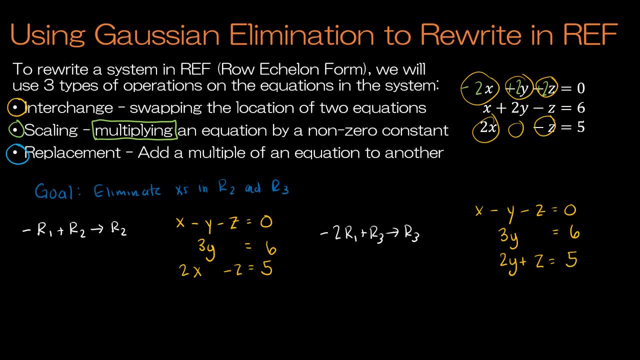 The second row, I want y, And now this one happened to get rid of z, but that's okay. But the last row, I want only z. So how am I going to get rid of z? I'm sorry, How am I going to get rid of y in the third row? 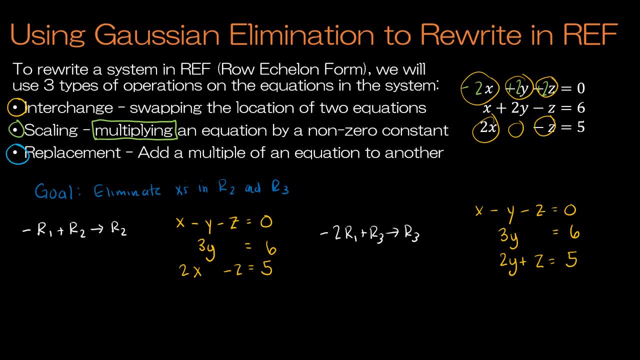 Now I wouldn't want to use row 1, because, as you can see, if I did anything with row 1, I'm going to end up with an x back in row 3, and that's going backwards. So keep in mind that when I'm doing this next step, 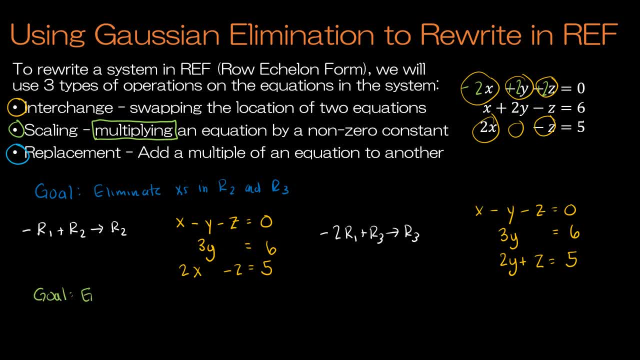 which is goal- eliminate y in row 3, I'm only going to be looking at these two. So how could I use these two equations? How could I use row 2 to eliminate the y in row 3?? So if I took yes, you're going to have fractions. 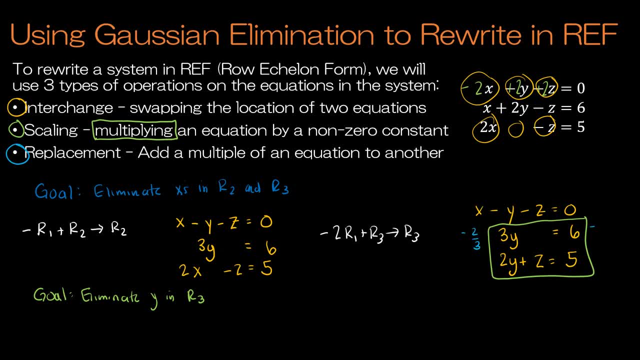 if I took negative 2 thirds times everything in row 2, what would I end up with? That would give me negative 2y. Well, that's what I want, right? I want negative 2y. So if you need to write what that new equation would be, 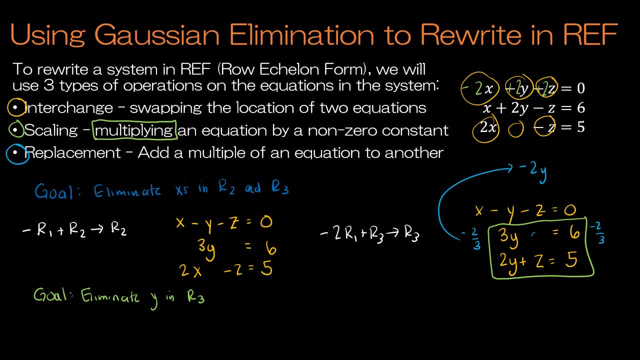 Negative 2 thirds times 3 is negative 2y. Obviously there was a 0 here, so that's not going to change. And then 6 times negative 2 thirds is going to give me negative 12 thirds, which is negative 4.. 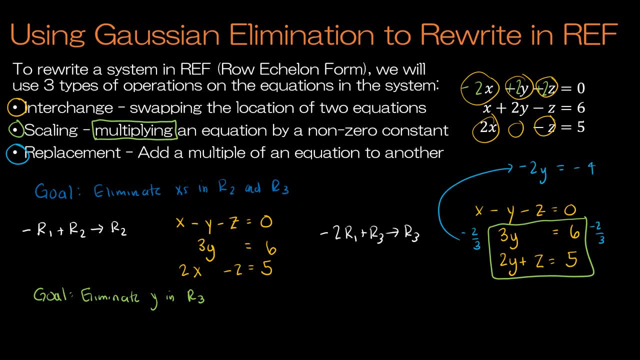 So I'm going to take negative 2 thirds times, row 2 plus row 3, to be my new row 3.. This is how we write that. I am a stickler about this, so if you are in my class and watching this video, 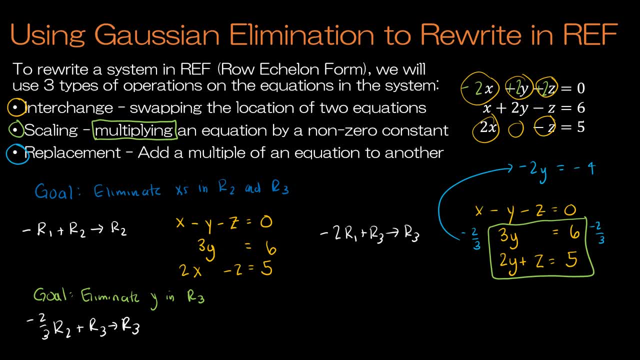 make sure that you are writing it in this way. Now, what is my new system? Did I do anything to row 1?? No, I've got x minus y minus z. oops, x minus y minus z is equal to 0.. 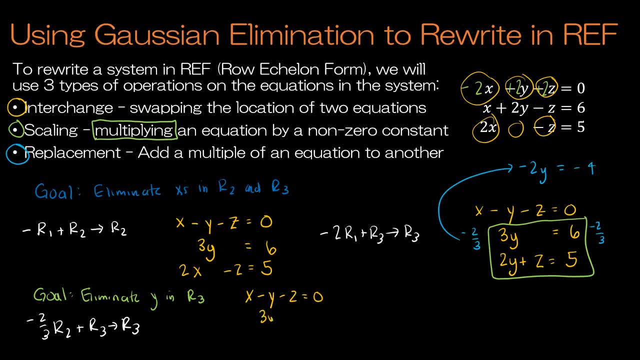 What's my new row 2?? I didn't change row 2.. I have 3y is equal to 6.. What's my new row 3?? Well, negative 2y plus 2y, that's no more y's. 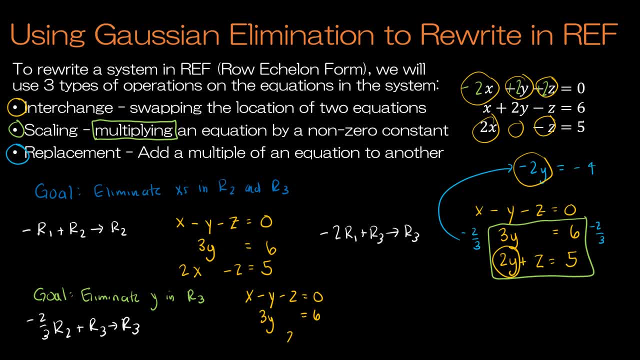 No, z's plus z gives me z, And then negative 4 plus 5 gives me 1.. So now I'm going to solve, because now it's in row echelon form, So I'm going to use back substitution. So here's my system of equations. 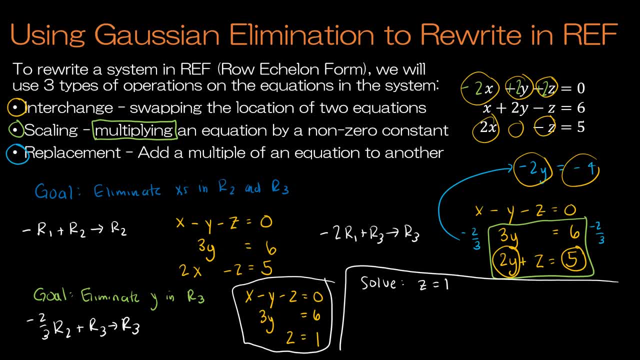 I know that z is equal to 1.. I already found that Solve for y. I don't even need to plug in z, I just divide to find that y is 2.. And then to find x, x minus y, which is 2,. 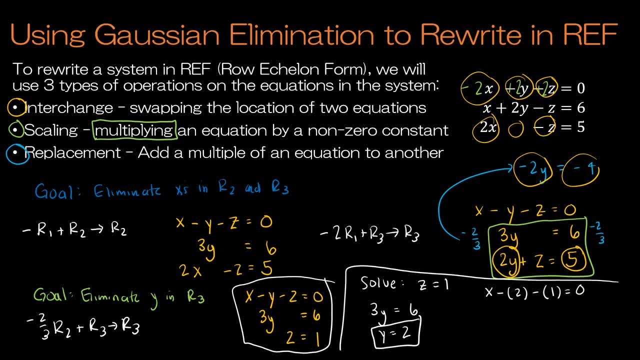 minus z, which is 1, is equal to 0.. So x minus 3 is equal to 0. So x is 3.. So what's my solution? My solution is: x is 3, y is 2, z is 1.. 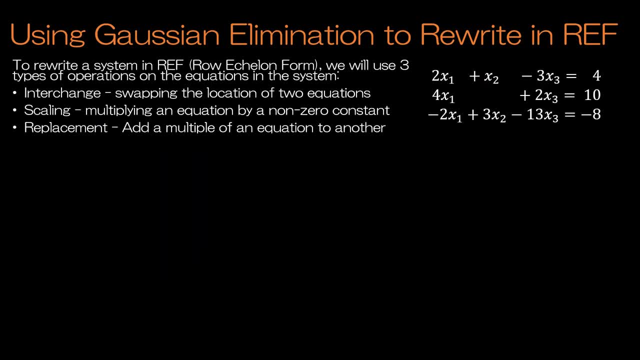 That's my final solution. We're going to do another practice together. Keep in mind, the practice that we just did a moment ago gave us just one solution. So if you'll think back to the beginning of the video, where we said what are the options, 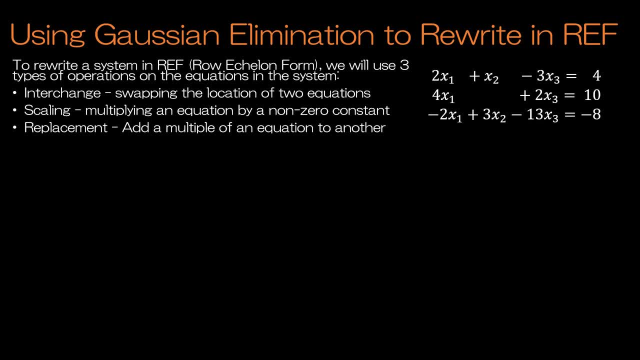 the options are: you get one solution, you get infinitely many solutions or you get no solutions. So we're going to do something here And it's not going to be one solution. It's either going to be no solution or infinitely many. 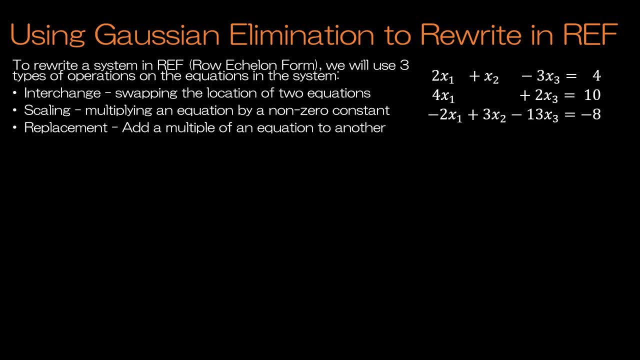 If you feel comfortable, start working through this on your own. We're going to start using the exact same steps. So my first goal is first to get rid of the x's in row 2 and row 3.. So if I start by looking at row 1 and row 2,, 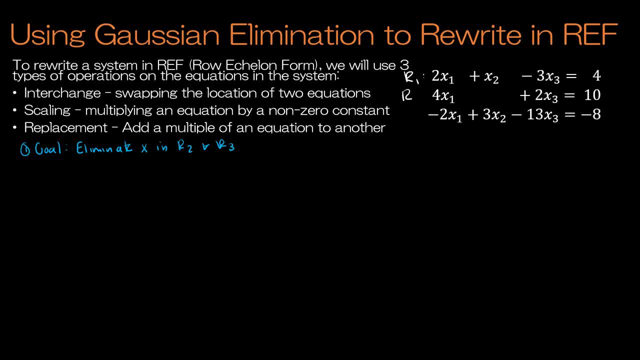 and again, feel free to label those row 1,, row 2,, row 3.. The first thing I want to do is get rid of the x here. So how can I get rid of 4x1?? Well, I've got a 2x1.. 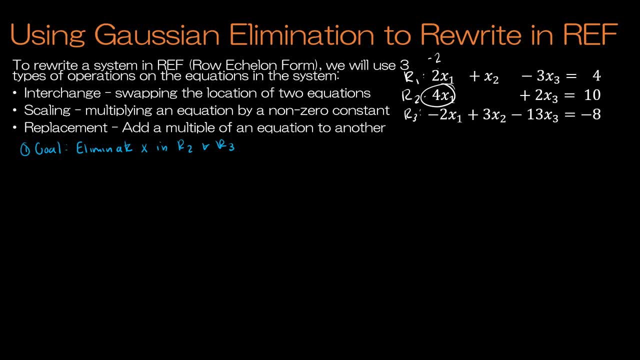 So what if I just took this times negative 2?? So I'm going to take negative 2, row 1 plus row 2 to be my new row 2.. So after I write what is called my row operation, written in the correct format, 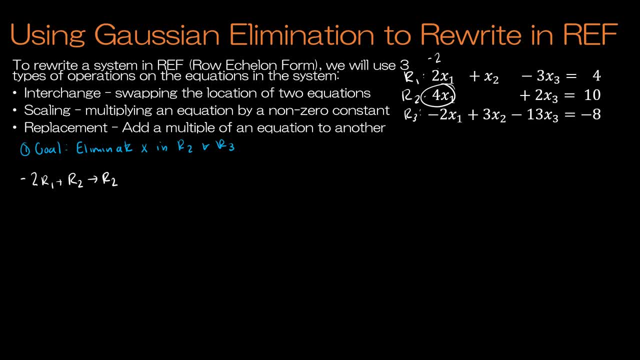 I'm then going to write what my new system of equations is. So did I change row 1?? No, not permanently. I'm just going to temporarily change it to get rid of that x in row 2.. What happens in row 2?? 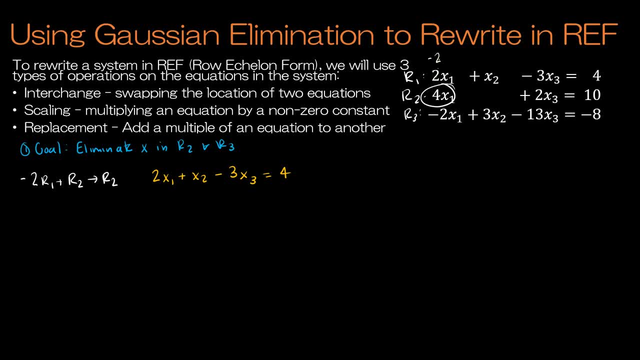 Well, if I took negative 2 times 2, that's negative 4x1, and this is positive 4x1, so the x1 goes away. Negative 2 times x2 is negative 2x2 plus 0.. 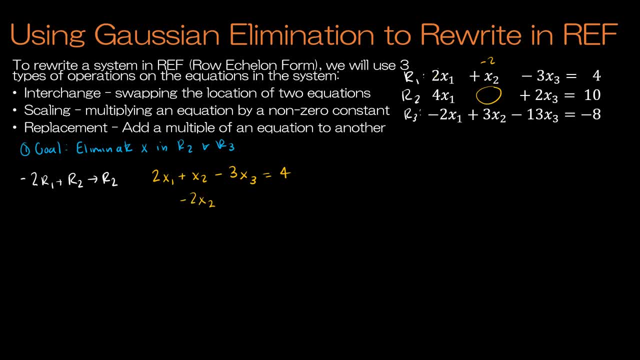 So that's negative 2x2.. Again, do as much or as little mental math as you're able. As much as you're able, Write it down. if you're not able, Negative 2 here would be positive 6x3 plus 2x3.. 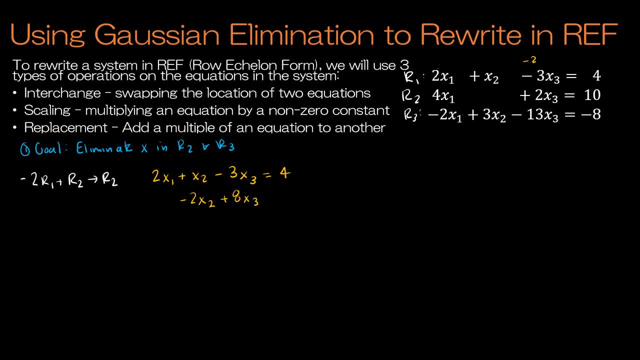 So that's positive 8x3.. And then again negative 2 here would give me negative 8 plus 10, which is 2.. And then did I do anything to row 3? No, I didn't. So I still have negative 2x1 plus 3x2 minus 13x3. 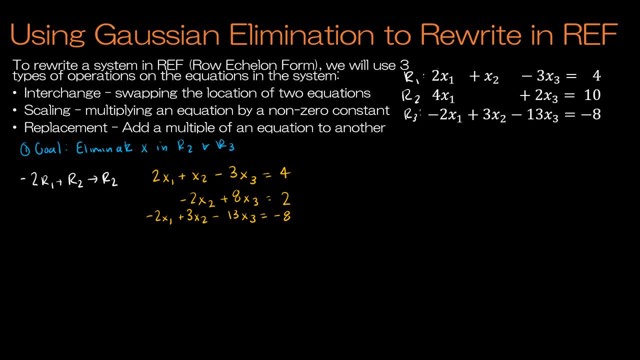 is equal to negative 8.. I still haven't eliminated the x in row 3, so now I'm going to do that. So, looking at row 3, I could really just add those two together. So that's what I'm going to do. 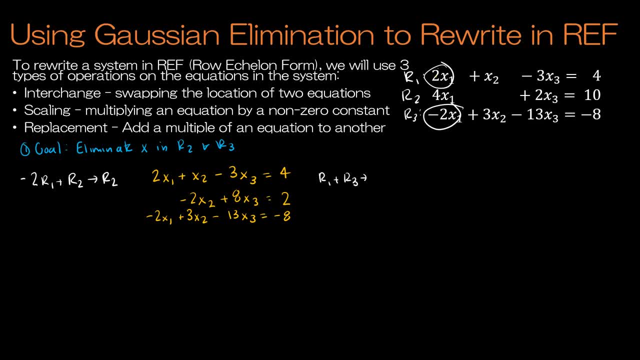 Row 1 plus row 3 is my new row 3.. So row 1 didn't change. 2x1 plus x2 minus x3 is equal to 4.. You might be saying, wow, can we just not keep writing everything? 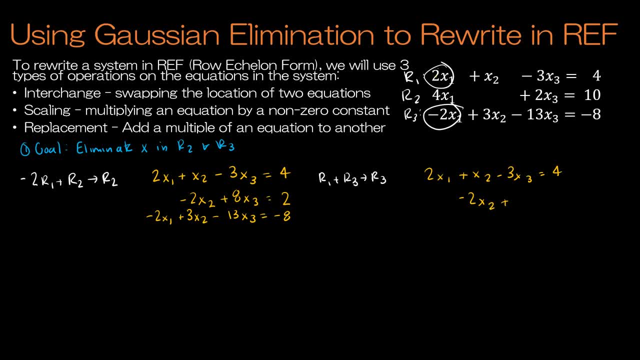 And the answer is no, You have to keep writing everything. So again, if you're in my class and you're trying to half-ass it and not write all of the equations, I'm going to dang you for that. So don't do that. 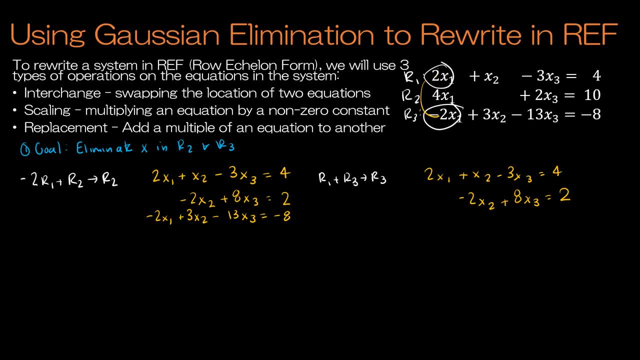 Now I'm going to add these two together, So 2x and negative 2x gives me 0.. x1 is gone. That's what I wanted. x2 and 3x2 gives me 4x2.. Negative 3 and negative 13 gives me. 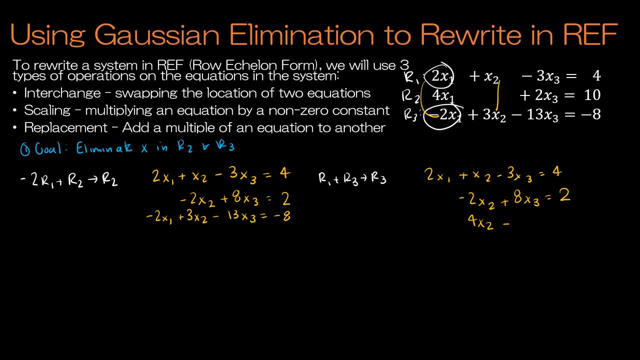 negative 16x3,, so minus 16x3.. 4 and negative 8 gives me negative 4.. So this is where I am now. This is my new system. Now, what's my next goal? So my next goal is to eliminate y in R3,. 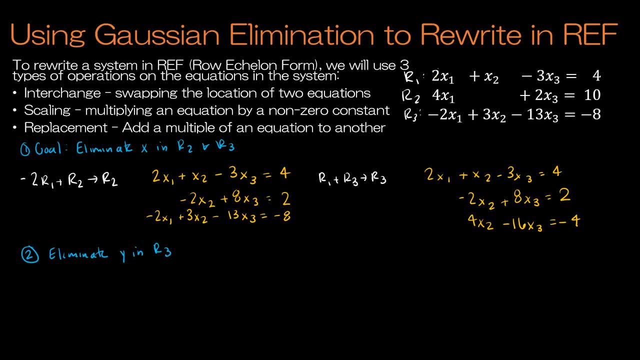 just as we did before. So I'm trying to get rid of y, which of course, is really just x2.. So I'll change that to x2.. Sorry for any confusion I caused there. So I'm trying to get rid of x2.. 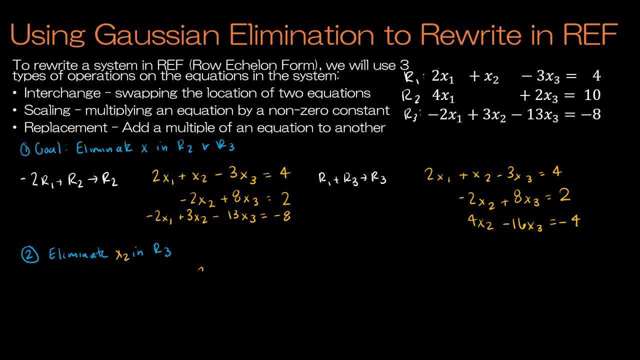 So what's going to happen? Well, this guy is not going to change, So I'm going to go ahead and rewrite it. And actually R2 is not going to change right. So now I get x3.. How am I going to get rid of this guy? 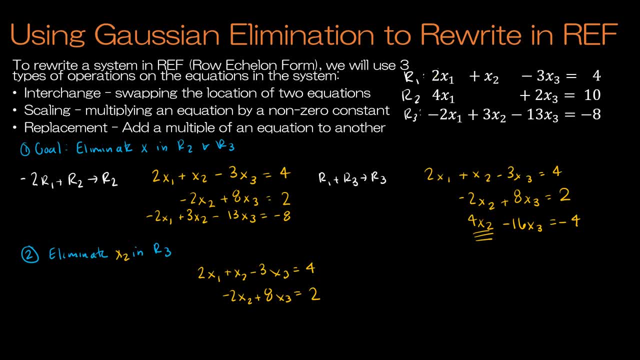 In x3?? Well, it looks like I could just take 2 times R2, which would give me negative 4x2, and add it to the 4x2 on R3.. So 2 R2 plus R3 is going to be my new R3. 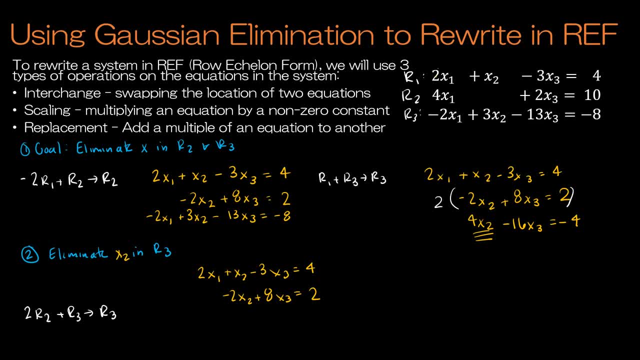 What does that leave me with? Well, that's negative 4x2 plus 4x2.. Those are going to go away. And then 16x3 plus negative 16x3.. Those are going to go away. So I have 0.. 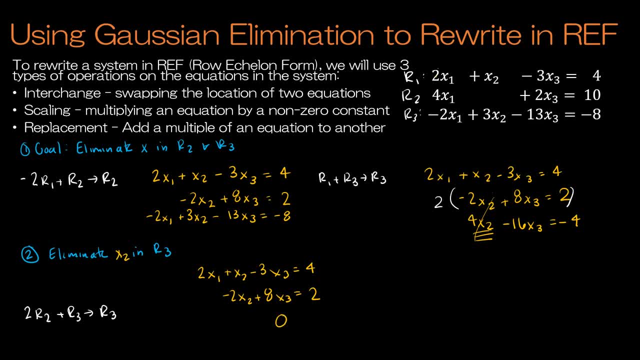 And then I've got 2 times 2.. That's 4 plus negative. 4 equals 0. This is really important. So please pay attention to this. What just happened is we essentially had the same equation twice, because when I combined them together, 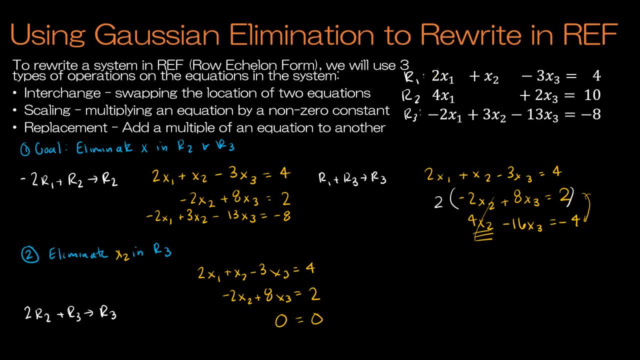 one of them disappeared completely. Now, if you'll recall, three options: First, one solution. That's not this case. Second was infinitely many solutions, And that's when you had the same equation twice. So that's what's going to happen here. 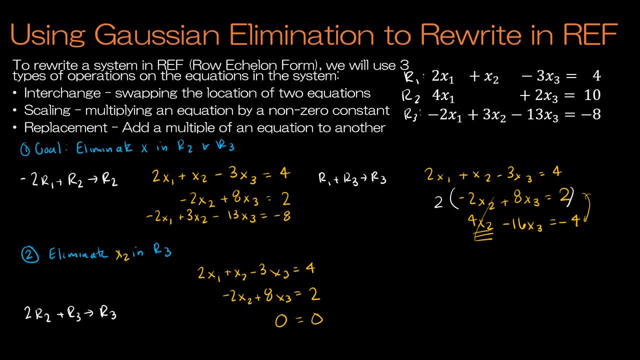 This is going to be consistent. But because this is true, then we have a free variable. So we're going to say- I'm just going to write it here, so you remember, x3 is free And that means we're going to have: 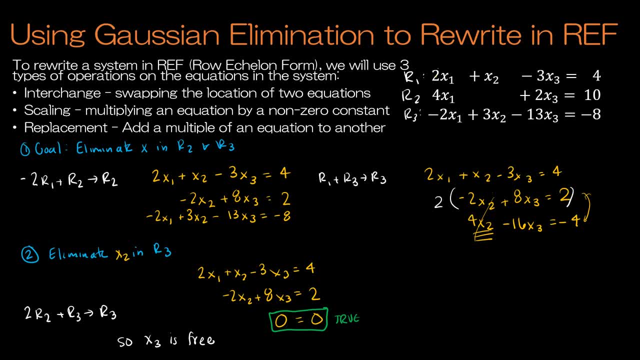 infinitely many solutions, But we want a way to describe what those solutions are, Again parametrically. So I'm going to let x3 equal t Or t equals x3.. So we're going to write it with respect to t. 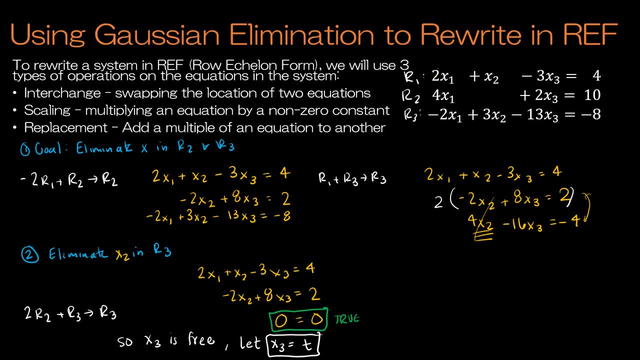 So when we write our final solution, we're going to write it with respect to t. So now I'm going to solve For x2.. Which would be solving for y. basically, I have. If I'm solving for y, I'm going to take. 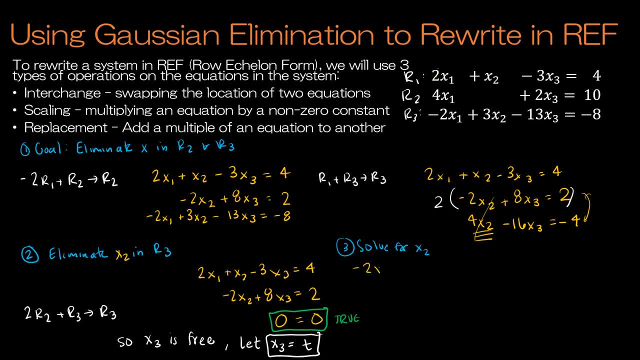 Two sorry Negative: 2x2 plus 8x3.. Is equal to 2.. But I'm going to replace x3 with t, Because that's what I just said I was going to do right here. So now, instead of 8x3.. 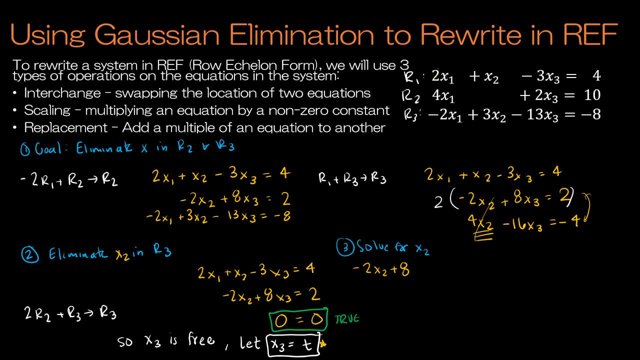 I have 8t Equals 2.. Now all I want to do is Rearrange that To get x2 by itself. So negative 2x2. Is equal to 2 minus 8t. Divide everything by negative 2.. 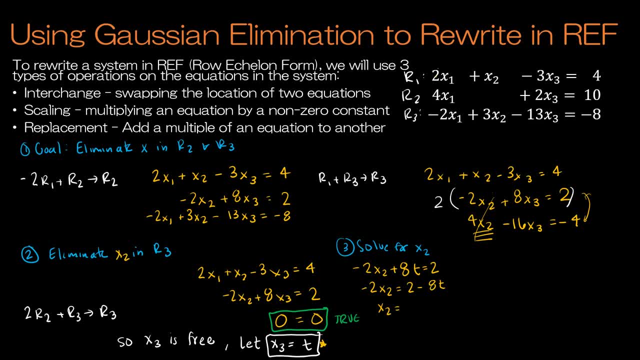 I get x2.. Is equal to 2. divided by negative, 2. Is negative 1. And then negative 8.. Divided by negative 2. Is positive 4.. So I can leave it like that, Or I can say: x2 is 14 minus 1.. 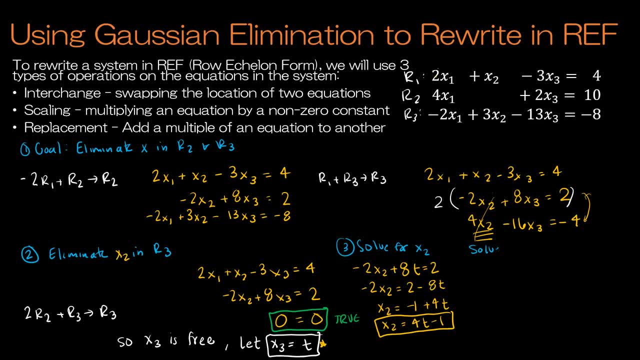 And then I'm going to solve For x1.. Doing the exact same thing that I did before. This one's going to be a little bit trickier, So I'm going to have my Row 1., Which is 2x1.. 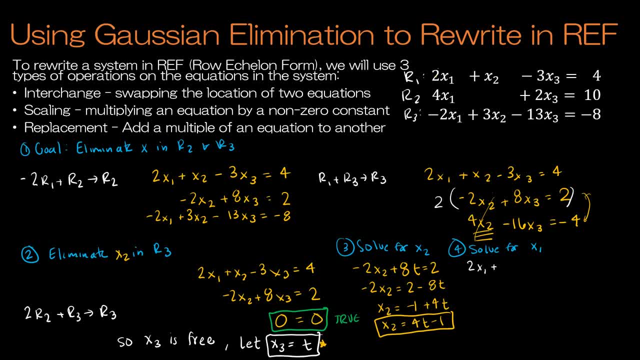 And then plus x2.. But x2. Is actually 4t minus 1. And then minus 3x3.. Well, x3 was t Is equal to 4.. So I just used this equation And replaced x2.. 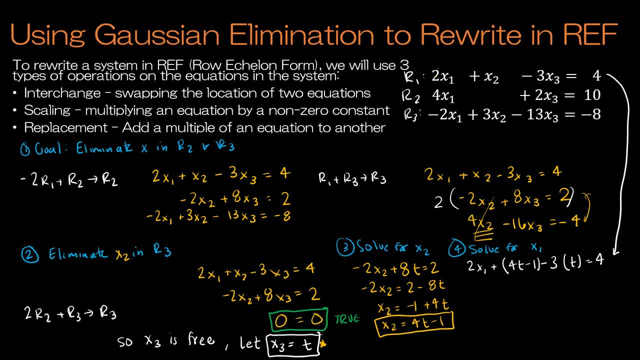 With 14 minus 1. And x3 with t. And now I'm going to simplify. So 2x1. Plus 1 minus 3t Equals 4.. I get 2x1.. 4t minus 3t. 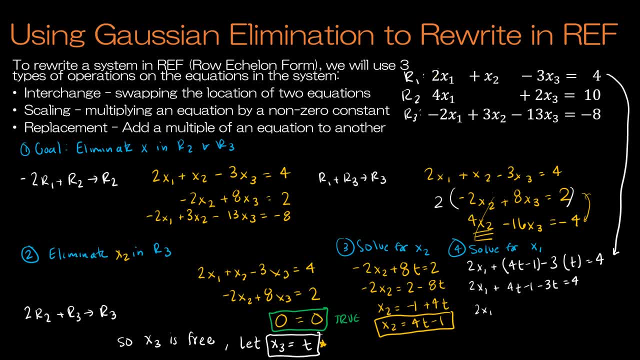 Is just t Whoops. So plus t minus 1. Is equal to 4.. Move everything to the opposite side, I get 5. Minus t, And then of course divide by 2. So I get x1.. 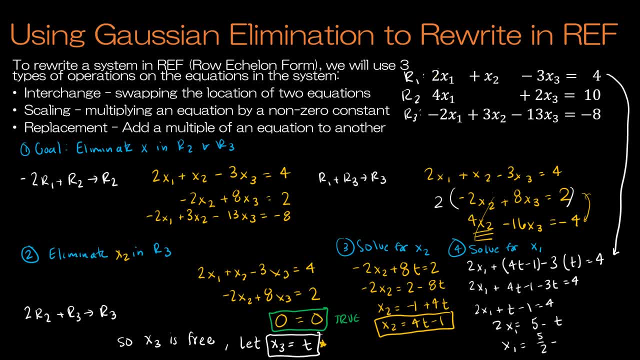 To 5 halves Minus 1 half t. Now I've obviously run out of room here, But The final solution Would be me writing 1,, 2,, these 3 things. So I would say the solution. 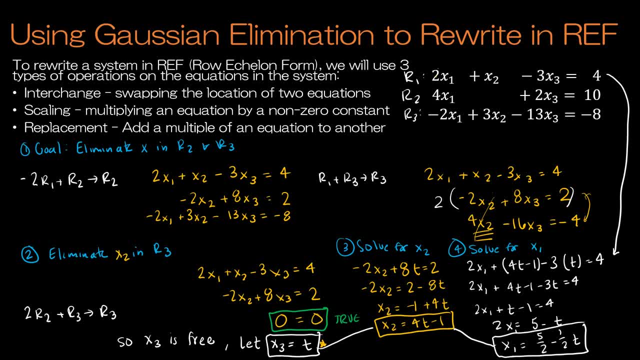 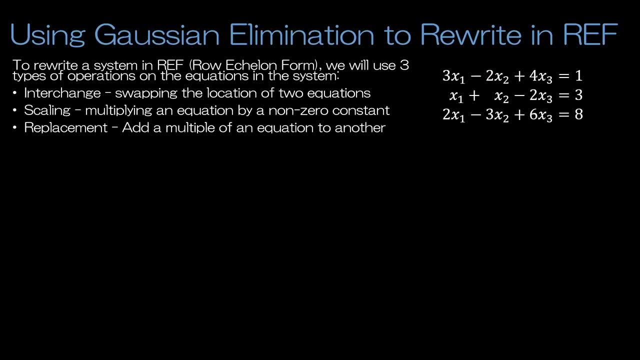 Is: x1 is 5 halves minus 1 half t. x2 is 14 minus 1.. And x3 is t Again, Because this one has infinitely Many Solutions, So we had to write the solution Parametrically. 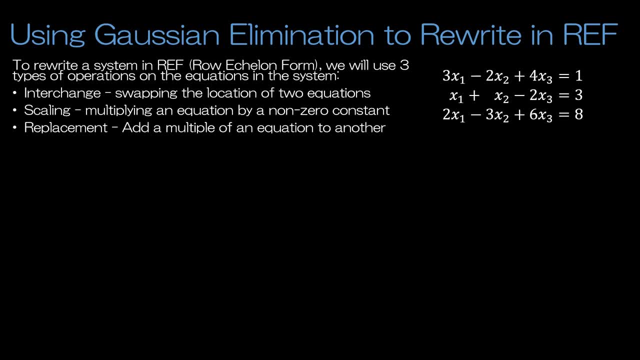 We do have one more question to do, And that question is Going to end up being An inconsistent system Because we haven't done one of those yet. I would like you to try this question on your own. Get as far as you can. 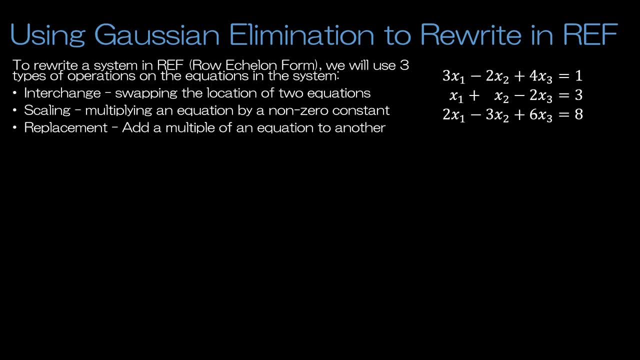 Until maybe something doesn't make sense, And then stop, And then we'll work through the rest together. Now, Again, There's three different Row operations that I can do, And there's more than one correct way to do this. So let me stress to you: 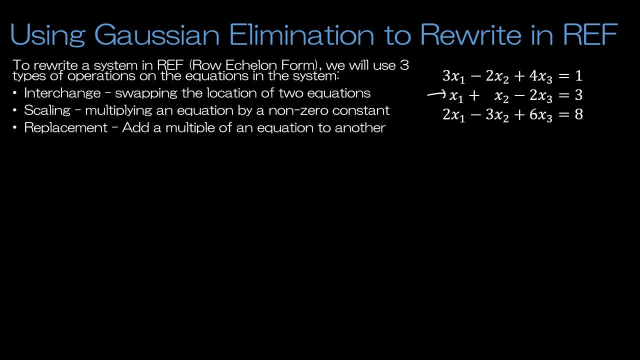 I'm going to start this question Because I like this guy to be My first row. I'm going to start this question doing an interchange. If you didn't do it that way, That doesn't make it wrong What I knew would happen. 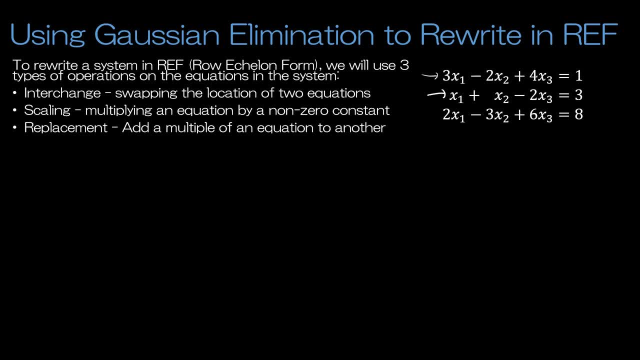 Is if I started working with this guy as row 1.. I would have a lot of fractions, And some people are really scared of fractions, So I didn't want to do that. So my first step, Or my first row operation, Is simply to swap row 1 and row 2.. 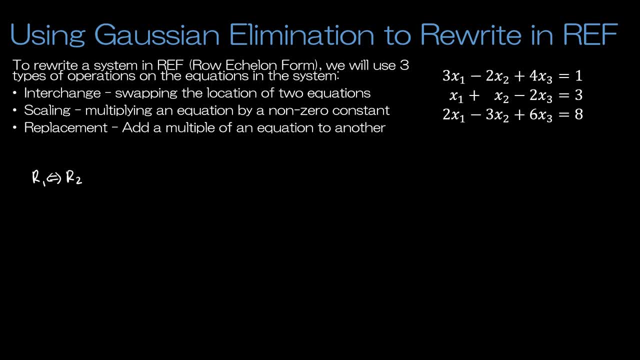 And the reason for that, Again, Is so that my first row Is now x1 plus x2 minus 2x3.. Is equal to 3.. And my second row Is now 3x1 minus 2x2.. 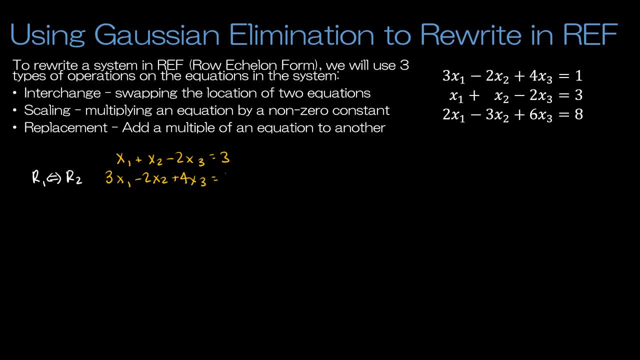 Plus 4x3.. Equals 1.. And I didn't do a darn thing to row 3.. It's exactly as it was before. From here, I'm now going to work with What is a much easier thing to deal with. 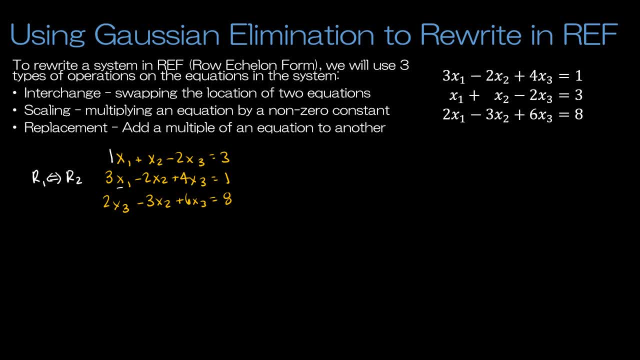 Which is 1x1.. To start getting rid of the x1's. I don't know where that 3 came from. Try to get rid of the x1's In row 2. And in row 3.. So let's see what my next step would be. 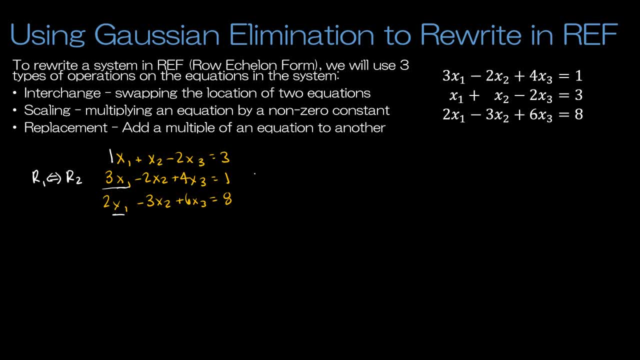 If I'm trying to get rid of 3x1.. I'm going to take Negative 3 times row 1. And I'm going to add it to row 2. To give me my new row 2.. So My first row didn't change. 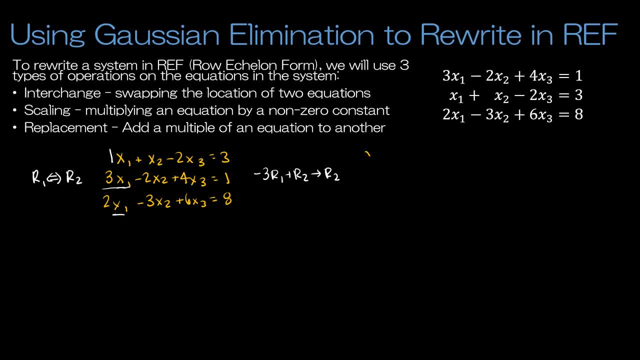 x1 plus x2.. Let's keep the same color scheme: x1 plus x2.. Minus 2x3. Is equal to 3.. Next one: I'm going to take negative 3 times this row And add it to row 2.. 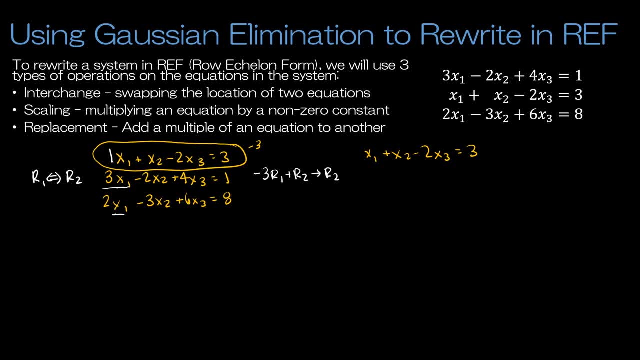 So that's negative: 3x1 plus 3x1.. Negative: 3x2.. Minus 2x2.. Is negative: 5x2.. Negative 3.. Times negative: 2.. Is positive: 6x3 plus 4.. 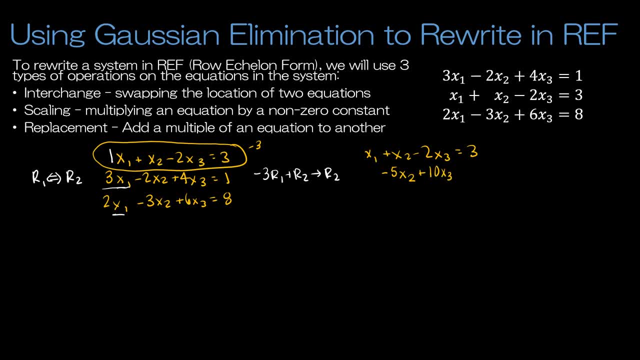 That's 10x3.. And then negative 9.. Plus 1 is negative 8.. I didn't do anything to row 3. So I'm just going to rewrite it. Now. you might be asking: Couldn't I just go ahead and do? 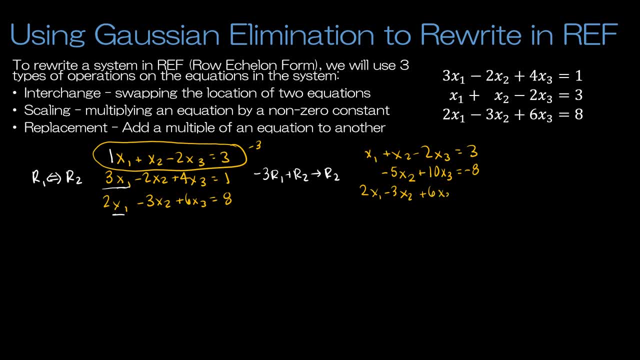 That next step for row 3 as well, And the answer is Eventually, But for now I want to see all of your work very clearly. So now Let's get rid of 2x1.. How am I going to do that? 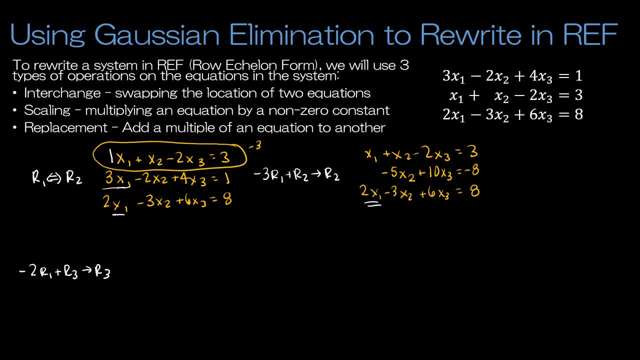 Take negative 2r1 plus r3.. To be my new r3.. So what happened to row 1? Nothing. x1 plus x2.. Minus 2x3. Is equal to 3.. What happened to row 2?? 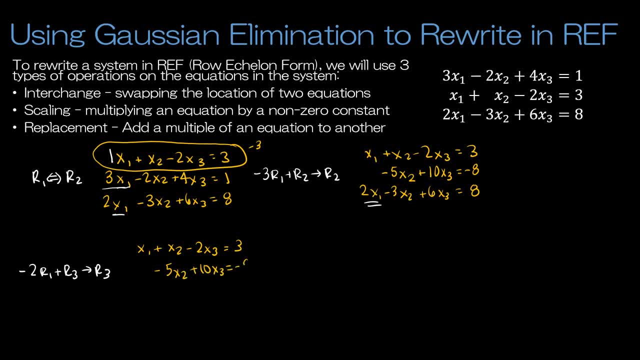 Nothing. And what happened to row 3?? I'm going to take This row Times negative 2. And add it to row 3.. So that's negative 2x1 plus 2x1.. No more x1's. 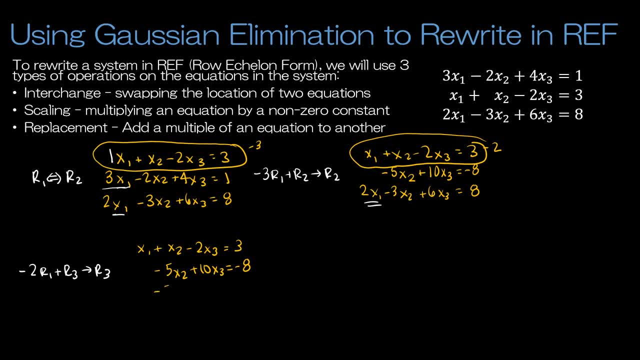 Negative 2x2 plus negative 3x2.. Is negative 5x2.. Negative 2. Times negative: 2. Is positive 4x3. Plus 6x3. Is 10x3. And negative 2 times 3.. 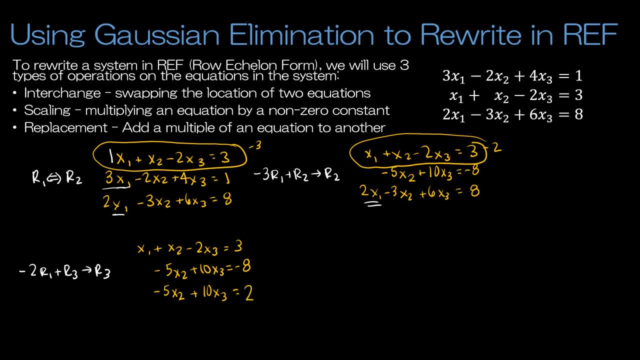 Is negative 6 plus 8. Which is positive, 2.. Now Hopefully you can see a problem right here. I've got the same two equations twice And they equal different things. But let's just make it very clear: Negative r2 plus r3..